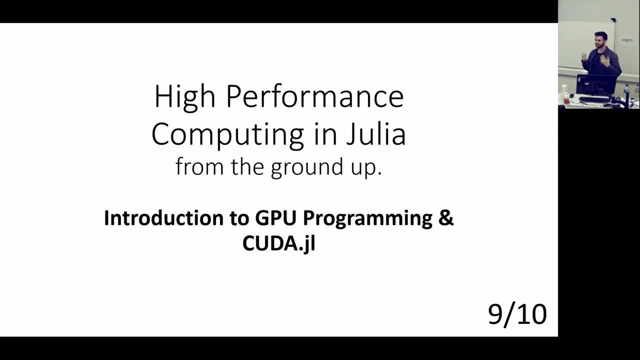 Okay, thank you everyone for coming. So this is the last week of teaching. So today we'll just go over a sort of introduction to GPU programming. We'll go back to where we started at the beginning and talk about the actual hardware itself, And then on Thursday, the next session, we'll talk 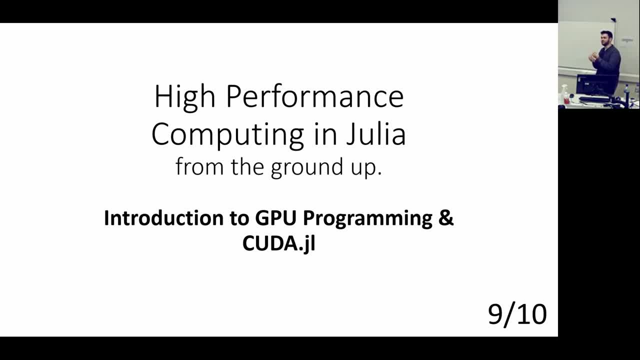 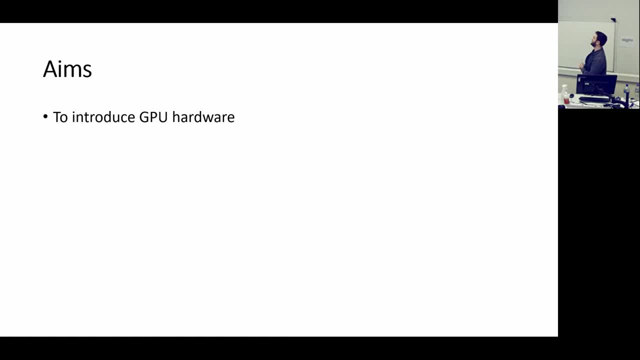 about the sort of nitty gritty of programming these devices. So today what I want to talk about is just first sort of introduce the actual GPU hardware, in case some of you aren't familiar with it, to talk about the sort of different options we have when we're programming. 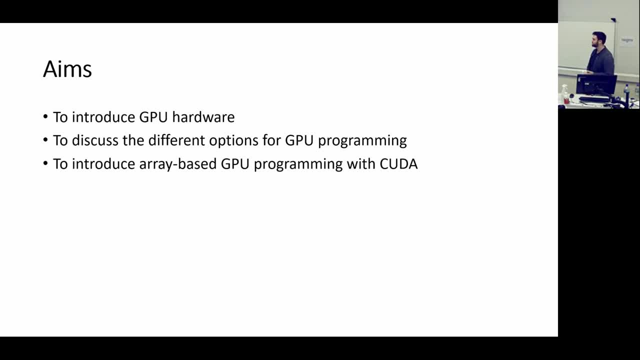 for a GPU To introduce a sort of array-based way of programming with a GPU. this is quite similar to how you would use like NumPy with Python and you sort of abstract away a lot of the complexity and just call sort of generic array level functions. 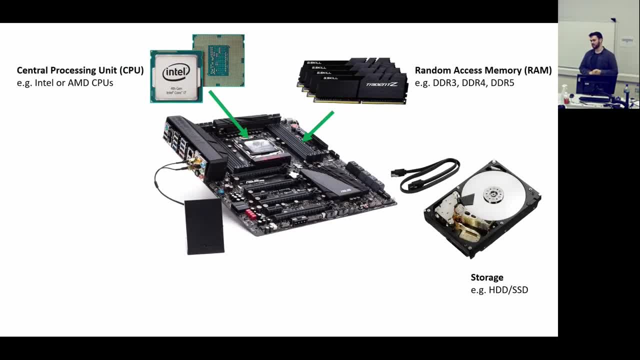 Okay, so this is the sort of picture that we built up last time in well, actually at the start of the course. So, as a sort of recap, you have the motherboard, which is the image in the center which connects all of your different devices together. So you have some. 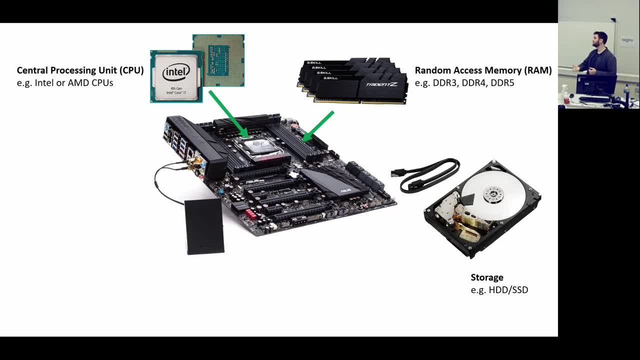 permanent storage and like a hard drive, you have some random access memory. that sort of is your, your sort of working memory while you're processing things, and you actually have the sort of brain of the computer itself, The processor, But optionally you could also have a graphics card, So this is like a separate 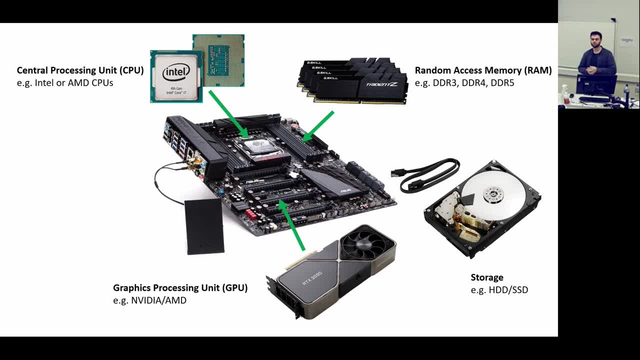 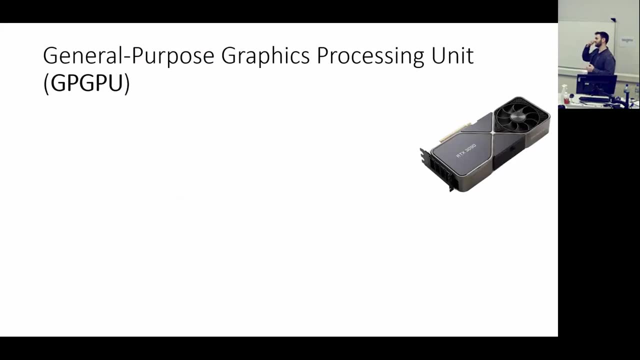 device that you can add into your computer to sort of offload a few specialized workloads that can be processed more efficiently on a GPU over a CPU. So nowadays the companies that create these GPUs tend to call them GP GPUs, which is a kind of a generic GPU. but 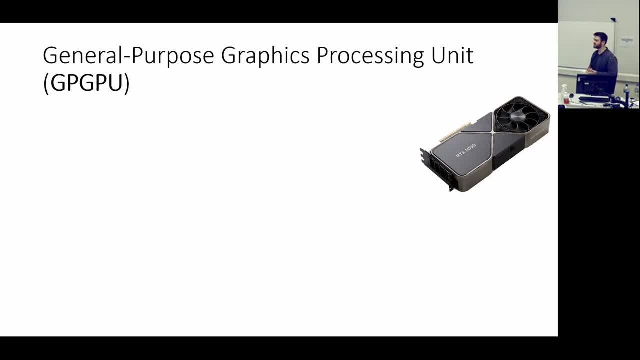 it's a kind of a general purpose graphics processing units, Because originally they started as specifically graphics oriented workloads, So sort of rendering, sort of pixels to a screen on a game, or maybe it's from like an animation studio. that's like rendering. 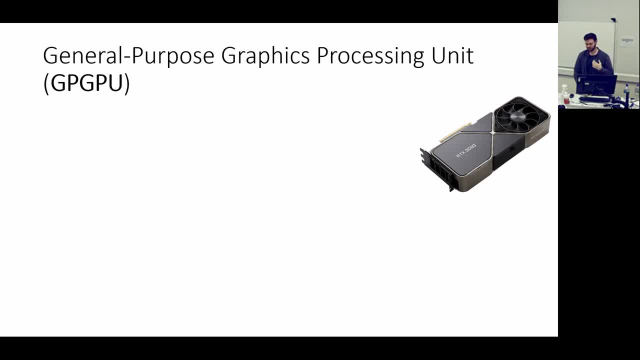 out their, their film or movie. But nowadays they're used for a lot more than just those sort of specialist applications. So graphics- or you might buy a GPU and do no graphics work with it at all. So these sort of devices are aimed at sort of massive parallelism, So they're aimed to sort of work alongside. 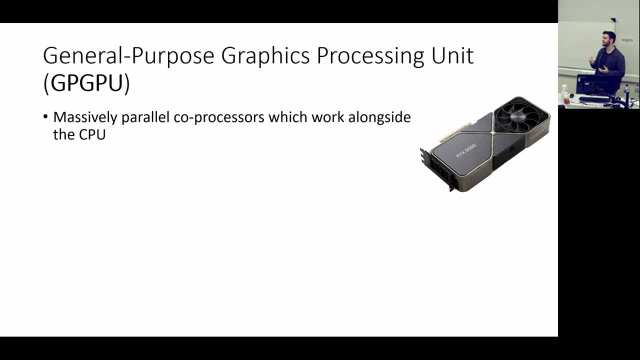 the CPU. while the CPU is sort of general purpose and can handle most tasks, The GPU is more designed for specifically highly parallelizable workloads, Additionally graphics workloads, But nowadays they're often used for other things, So they're really good at doing sort of big simulations, So like fluid dynamics. 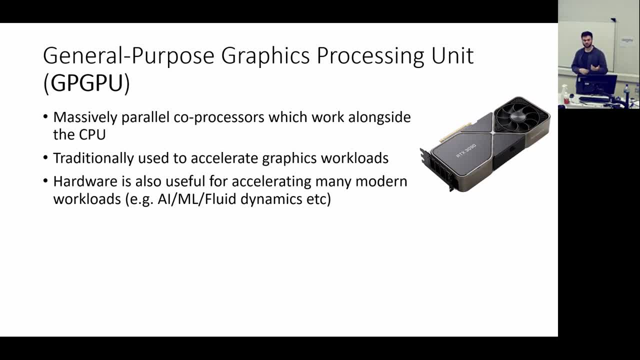 and stuff can be offloaded to a GPU. Also, if you're doing any sort of machine learning or AI, these are almost essential to actually be able to get the results you want in a sort of timely manner. These are the standard for AI and machine learning. So the main difference. 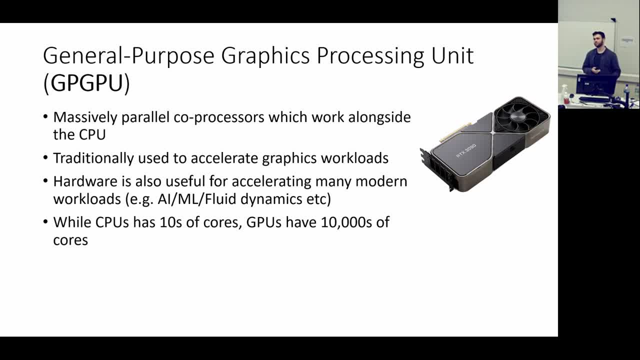 is well. a traditional GPU like the one in your computer might have sort of four, maybe eight cores. Some bigger desktops might have 16 or 32 cores. GPUs, at least the modern ones, have 10s of 1000s of cores working together. they have a slightly different structure, but the scales. 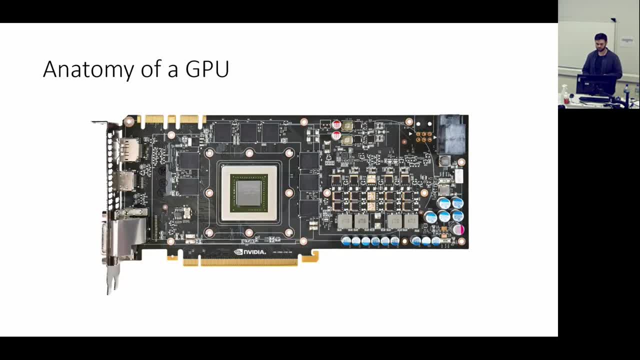 are orders of magnitude apart. So if we look sort of under the hood, if you look at a graphics card and take away all of the like heat sinks, this is sort of what you would see. So the one, the one part that's quite important is at the 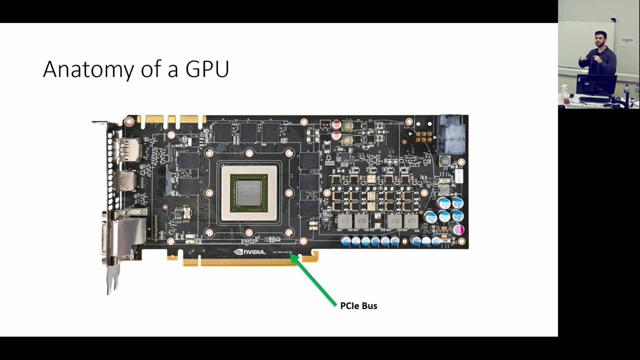 bottom there's a connector that connects it to the motherboard so it can communicate with your processor, And so these things work alongside each other to come up with a result. However, you'll notice these little sort of black chips and, scattered along the GPU itself, These 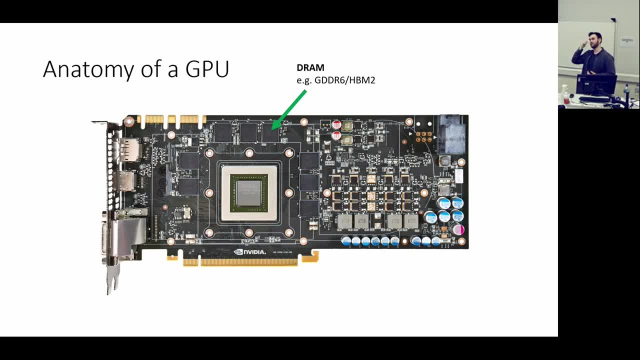 are memory chips, So GPU has its own memory. So, like you said, as you add a chip, you get memory that it works with. So you have your main memory, your RAM, which is separate to your GPU memory. And so if you were to actually see some sort of RAM chips, and they have these. 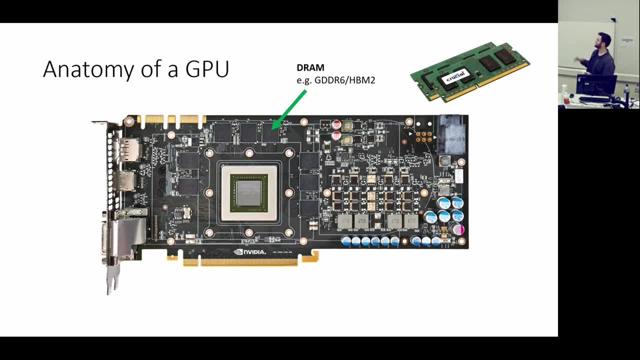 little black dots, these little black squares on them. they're very similar, But this memory tends to be a bit more specialized for what a GPU needs, So like high bandwidth instead of optimizing for latency. Also has its own power. So most of the cylinders that you can. 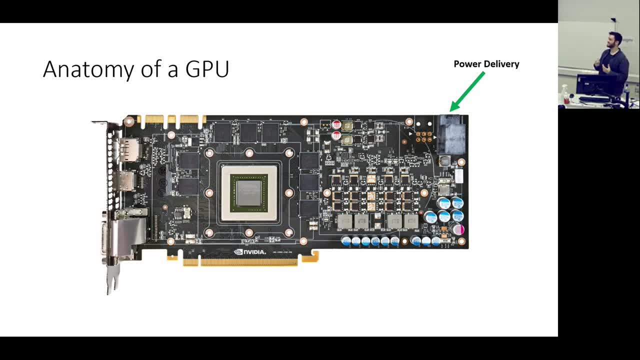 see on the card are just capacitors, So it is essentially like a self-contained computing unit. It has all the different parts on one chip And finally in the middle you have the actual processor itself. So if we zoom in a bit or use a diagram of the processor, 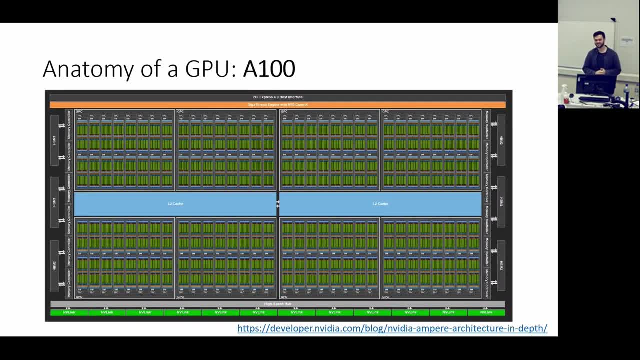 it can be a bit overwhelming to see what's actually happening. So this is an image taken from a blog post. NVIDIA did that sort of broke down one of their most recent cards, the A100.. This is the card that's available in Solus, the HPC. 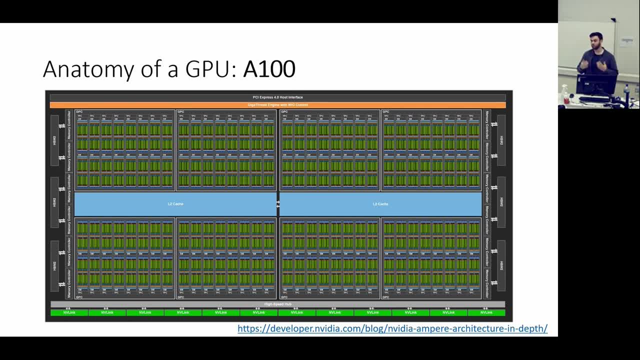 that we have access to here, or one of the HPCs we have access to here, And in this diagram I'll point out a few key points. So on the edges here you have these sort of modules. These are the little black chips that were on the previous slide. 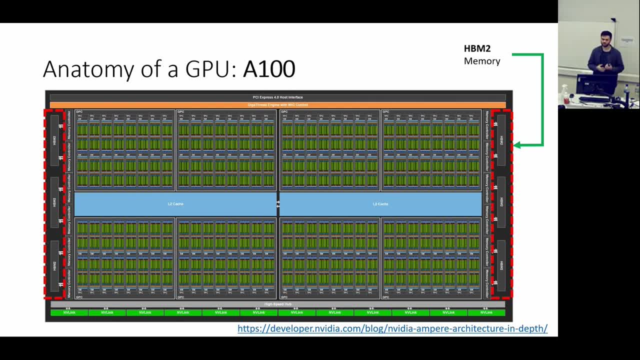 So it's basically just the onboard memory. So it's the memory that the GPU cores will have access to. Most modern ones use HBM2.. This just stands for high bandwidth memory, So it's very high throughput. That's all you really need to know about it. But what you 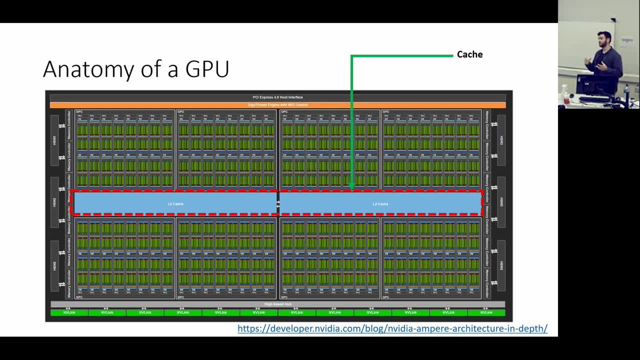 also notice is: just like the CPU, the GPU also has a lot of cache on board as well, And we sort of spoke a lot about cache and how important it is for the CPU, So you can make sure you can compute at the speeds necessary, because memory tends to be a lot slower than 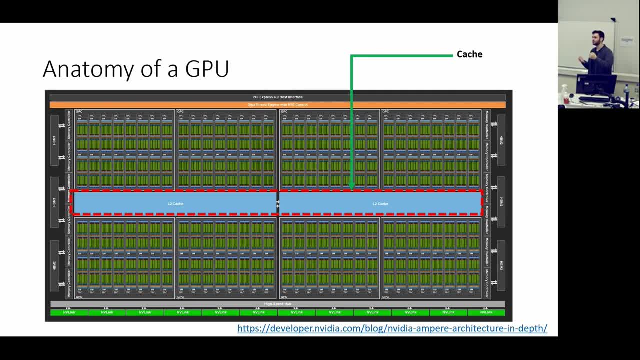 your actual clock, the actual clock cycles of your CPU. So you need to be able to have some really fast cache to be able to feed the processors so as to not bottleneck your calculations. And then these sort of little blocks here are on this diagram. They're not quite individual cores. 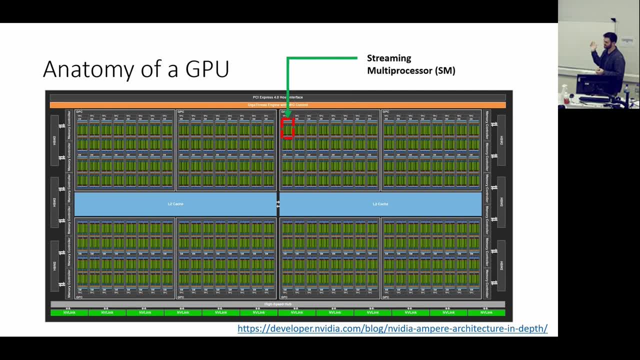 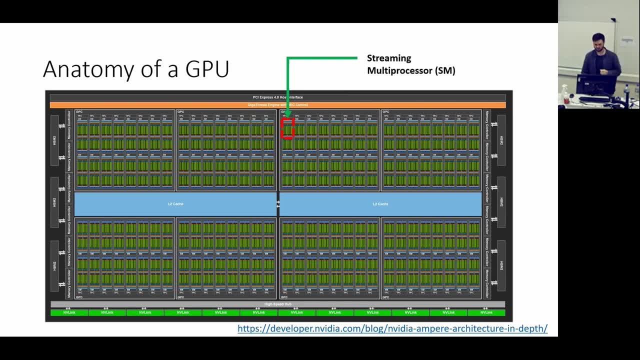 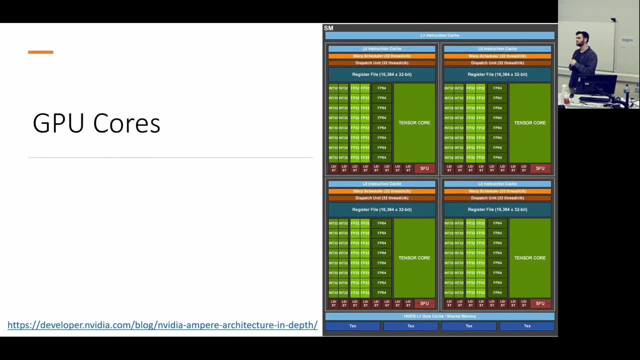 chunks of processors, So these contain multiple things. So again, zooming in once more, on the right we have a diagram of one of these streaming multiprocessors And you can see they have multiple cores throughout and they have specialized cores for doing certain operations. 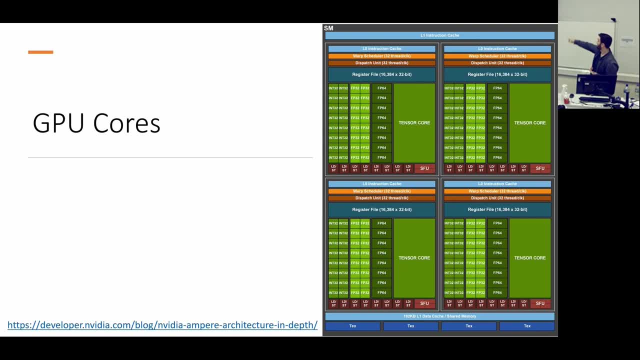 So, for example, you can see and sort of light-green, the small blocks, FP32, this is 32 bit floating point operations. So it has a special part of the chip just for doing those operations. It has a part for integers And it has a part for 64 bit floats. This is a modern GPU card. 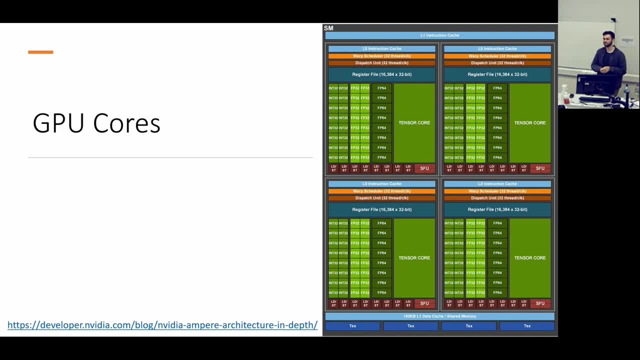 And so only the sort of higher-end, modern ones tend to have good support for 64 bit floating point operations. Because, again, these originally were designed for core. Because, again, these originally were designed for core. Because, again, these originally were designed for core. 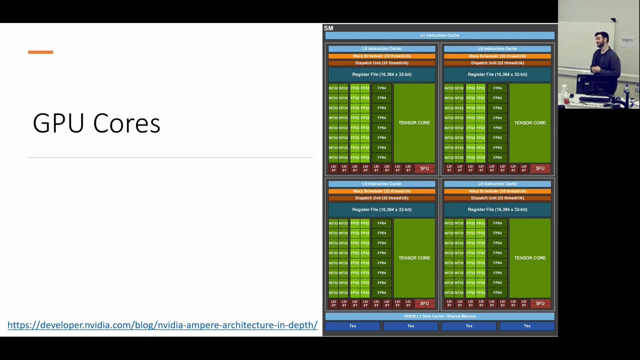 were designed for graphics cards and you don't really need high precision for graphics, whereas if we're doing sort of scientific numerical workloads we might need that extra position. so it's just important to sort of check whether the graphic card can actually support double floating point precision, which is the 64-bit type. Also, these new cores have huge sections which they 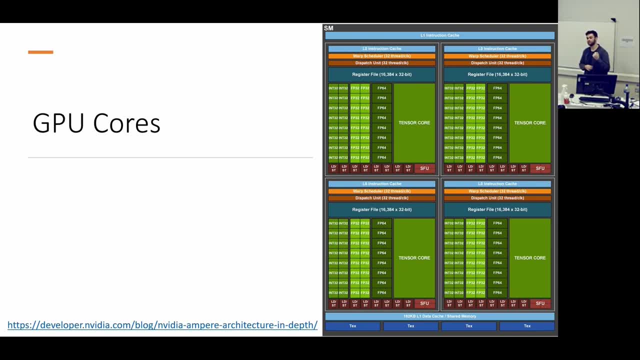 call tensor cores. These are like specialized cores for doing operations like matrix multiplication, because these come up a lot in loads of applications, specifically AI. So these tensor cores are really good for accelerating AI applications. So again, also what you can see here is there's lower levels of cache, so each of these cores has 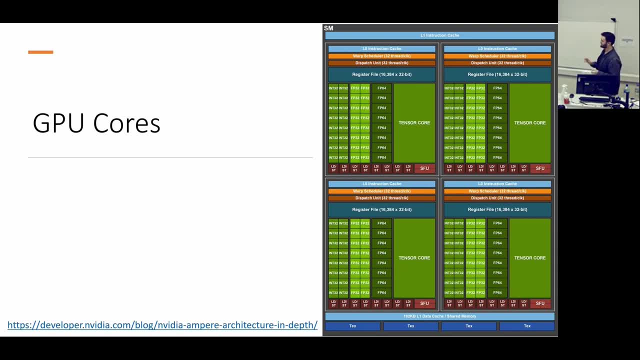 access to some sort of shared memory and hopefully what you can see from this is there are a lot and lots of cores so you can process lots and lots of instructions at the same time, But they're sort of suited more towards your typical sort of math operations. They're not as 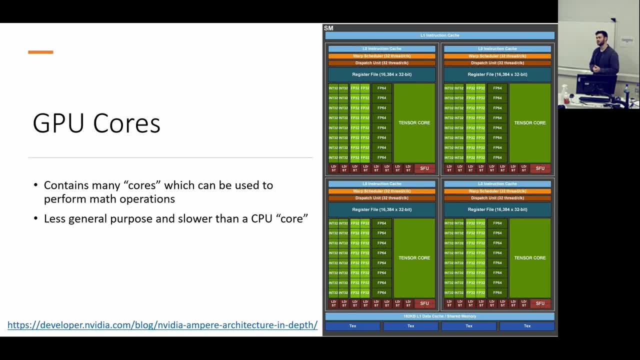 general purpose as what a CPU can do. A CPU is kind of like a jack of all trades: It can do everything and it can do everything quite quickly, whereas this is designed more for a specialized workload that is very high throughput, So you can do if a task is highly. 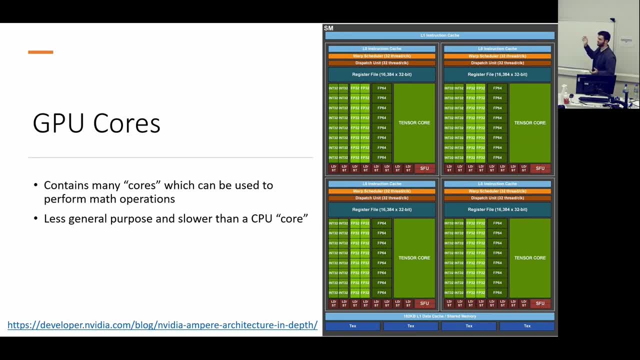 parallelized, it can do a lot of things, So you can do a lot of things. You can do a lot of things, But if it's feasible, you can do it on a GPU and if it's relatively straightforward. Also, something to notice is each core has access to far less cache than a CPU core. A CPU core 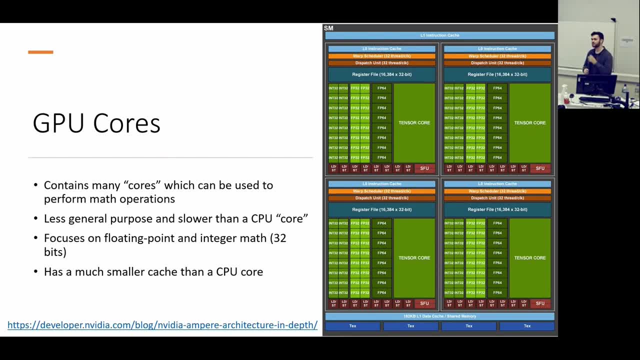 might have like 100 kilobytes of cache like per core. This is the cache right next to the CPU, Whereas all of all of the processors you see here have access to around 200 kilobytes and it's shared between all of them. 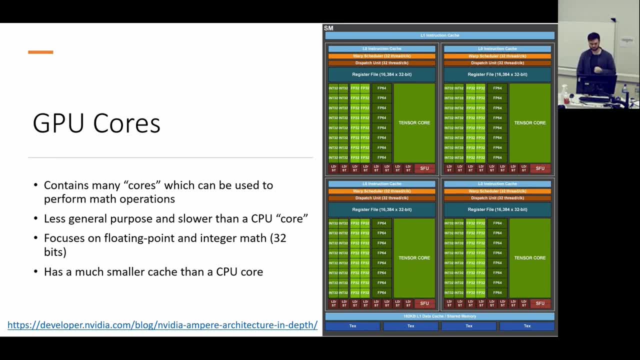 So what each core does has to use sort of less memory as well. Okay, great, Don't worry if you haven't taken all of this in. This is a more abstract notion. we might need it a little bit more next, on next Thursday. But all I want you to take away from 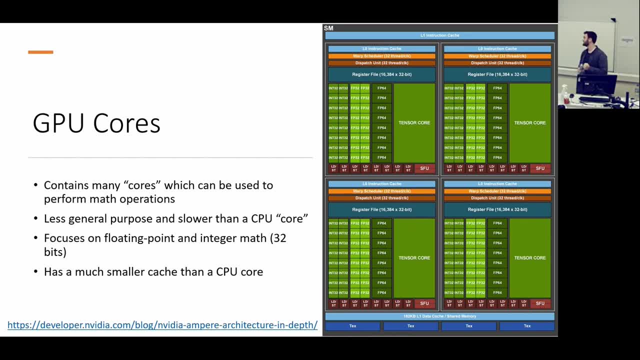 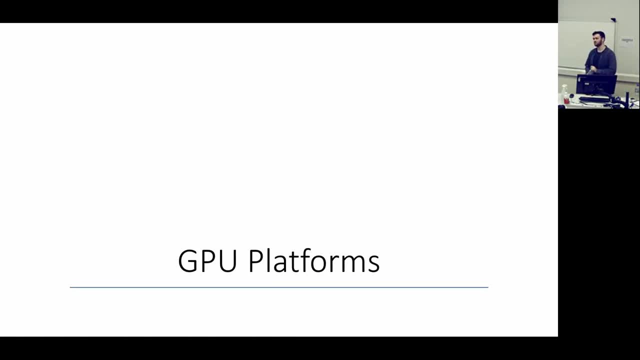 So we need to talk about some of the GPU platforms. So this is not the same as like, or it's a very different world to, CPU design. So CPUs, even if you, if you get your CPU from AMD or Intel, they use the same instruction set, and so we. 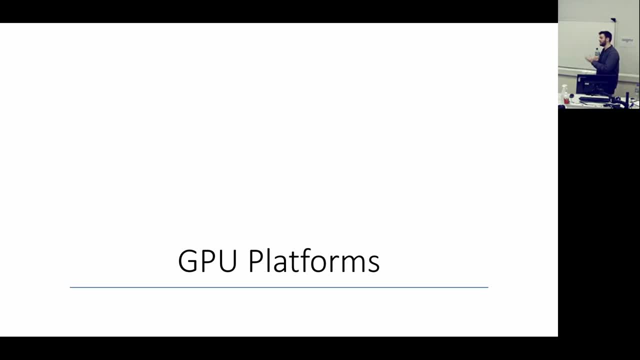 largely don't need to think about the vendor, so the manufacturer of the CPUs that we're using, Even ARM chips as well, like the M1, the Apple M1 chip. a lot of the instructions for that are abstracted away for us as programmers. 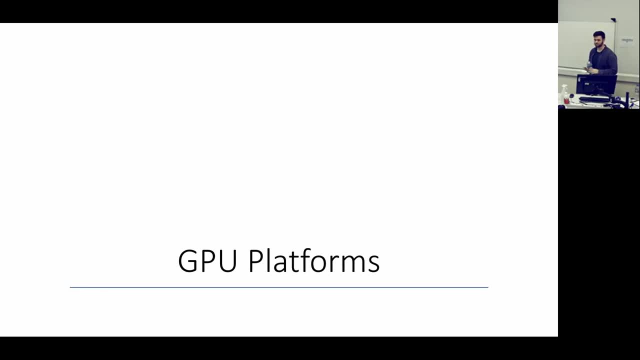 For GPU programming it's a lot more important which vendor comes up. So I've already named one vendor, NVIDIA, which is the sort of main one. Does anyone know any other vendors, any at all, that make GPUs? Yes, so ATI is the old name for the company that used to make a graphics card, but 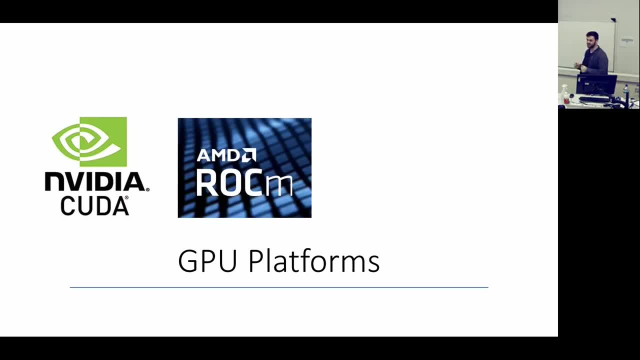 that got taken over by AMD. So now we have AMD as well. So they're the sort of second biggest, but I should really stress, NVIDIA have the vast majority of the market share, especially in HPC applications. So whenever you're using a cluster, it will probably be NVIDIA cards. 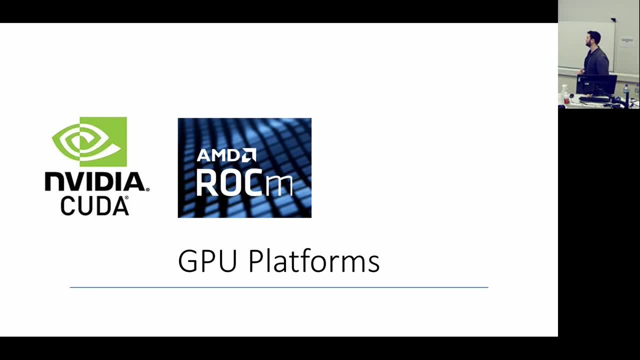 if it has GPUs. I should also mention that Intel are also trying to come into this and making their own GPUs, So I expect in the next few years they'll start making some data center oriented GPUs as well. They're not quite there yet, but it will probably come out in the future, So I mentioned it just. 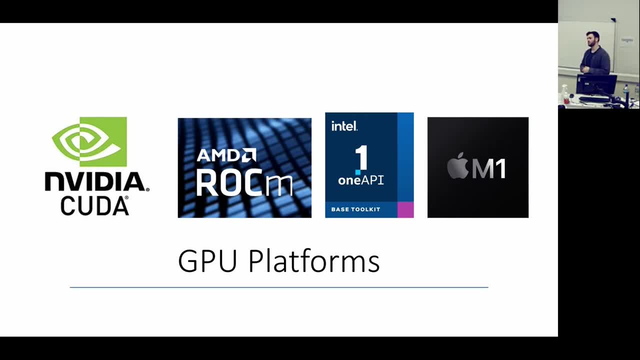 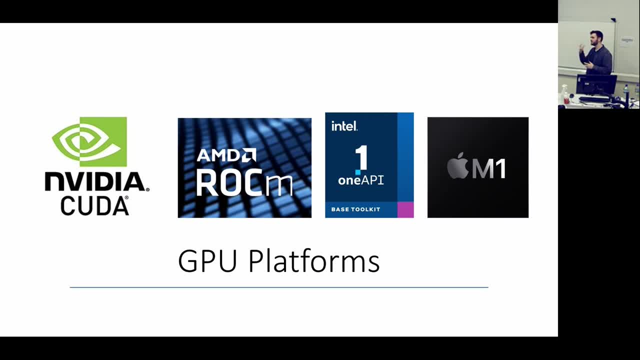 And they use something called metal to it's like a programming interface to program these GPUs. So what I'm going to focus on today, and also on Thursday, is talking about CUDA specifically, which is the sort of hardware platform and programming model that you use for NVIDIA GPUs. 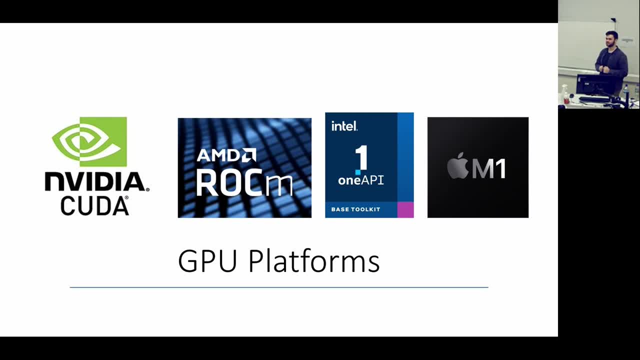 Unfortunately, CUDA only works on NVIDIA graphics cards and they've kept it quite closed- and yeah, it's very closed- so you can't run it on other platforms, Unfortunately. but there are other options that you can use and a lot of the skills are very transferrable if you have to learn another framework. 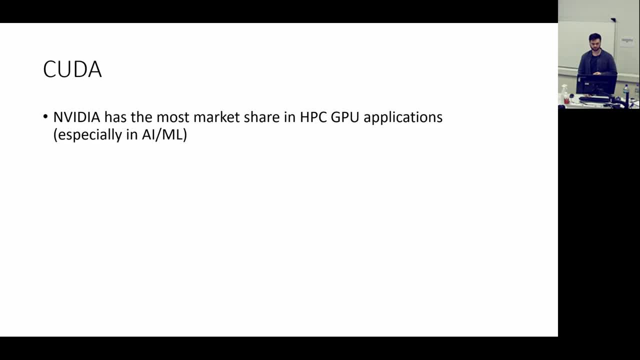 but just keep that in mind. So, yeah, So this CUDA is basically a sort of abstraction. It's a method that you can use to program for a GPU without having to think about the exact specifics of the graph, the particular graphics card you have, so each 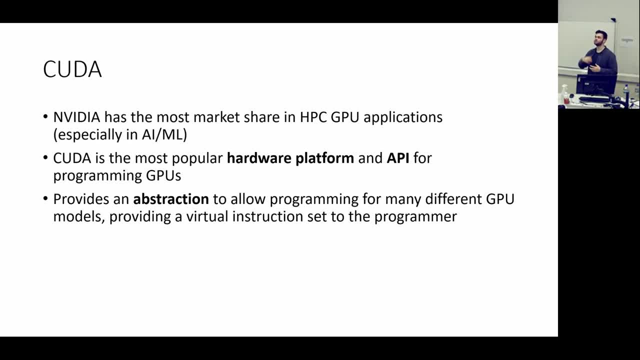 year they release a new generation and you don't want to have to rewrite all of your code to run on new GPUs. you want to be able to use your same code and compile it for the new graphics card and have it just work on there. and because from generation to generation there's a lot more. 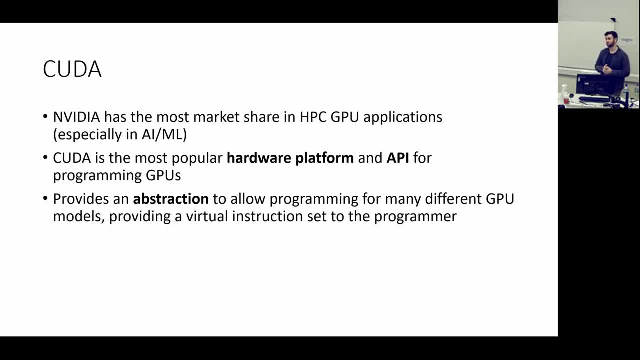 actual hardware changes under the hood that you would see on typical CPUs as well. so having this abstraction lets you write code that will sort of last a lot longer, Sorry, so CUDA also includes a bunch of like libraries written by the people at NVIDIA themselves that provide algorithms for doing your common stuff, so like BLAS, for example, which is: 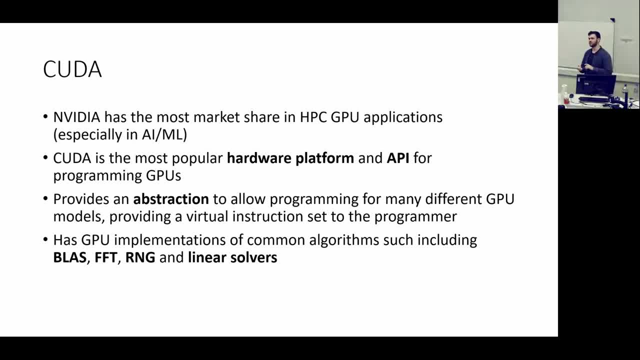 your basic linear algebra subsystems. so your matrix multiplies your dot products, sort of your generic operations like that. it also provides an interface for FFT, so fast Fourier transforms, which is also quite common and they're quite hard to implement yourself efficiently. so they give you some implementations. 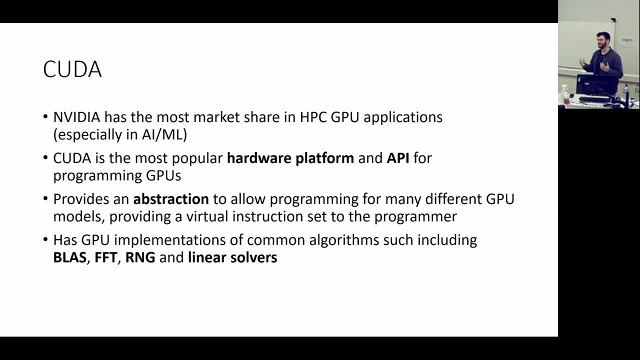 for that also random number generation and your typical math operations. so like sine cos, like exponentials, that will be implemented in the existing CUDA library. they also have quite a few linear solvers as well. so, for example, if you want to solve a set of simultaneous equations with like using a matrix. 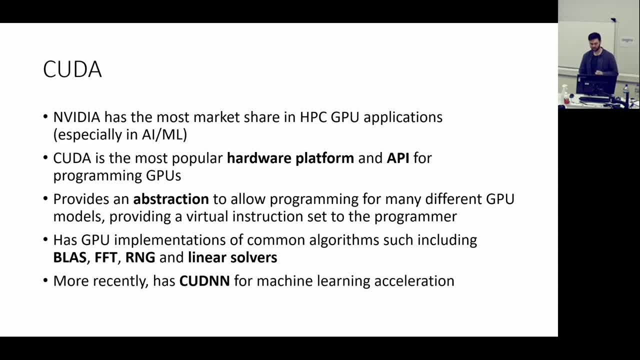 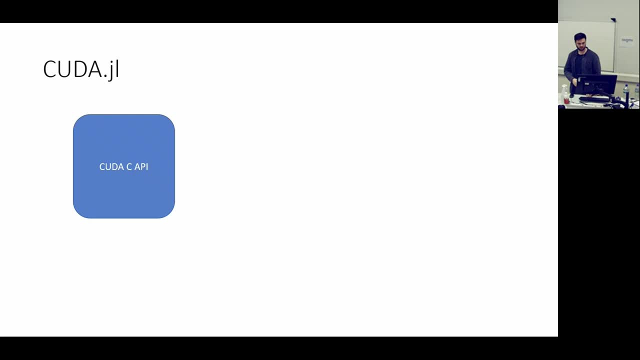 they have solvers for that as well. also, if you do machine learning or AI, you will probably have to install this additional cuDNN package which does sort of deep neural network accelerations as well. Okay, so CUDA originally is has um an API for languages like C and Fortran, because typically 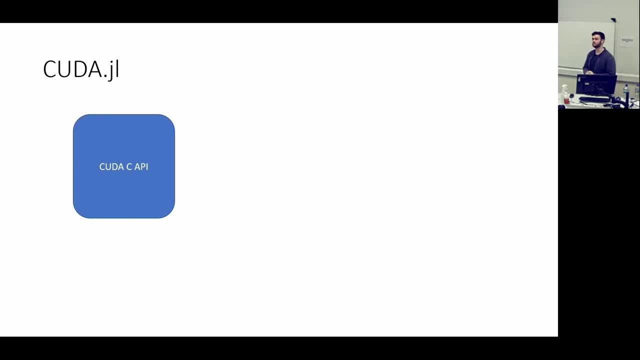 that's what sort of high performance programmers tend to use, and so we want to be able to make use of the C API. so a few people came along and created a package called CUDAjl, which sort of acts as a wrapper around the C API. 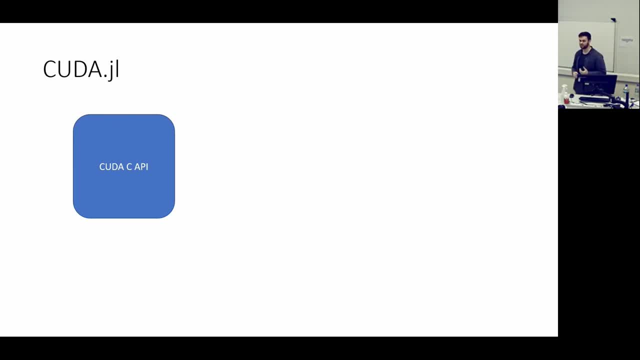 So we can use the functions from C without having to sort of re-implement everything from scratch. so this CUDAjl sort of sits on top of the, the C API, and essentially what that provides is some interfaces, some wrappers around the code so that we can use it natively from Julia. 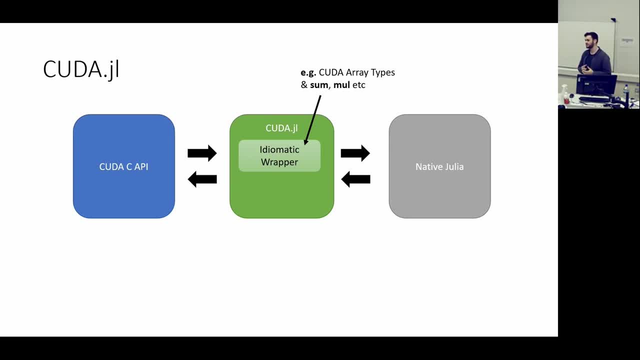 So the way it does this is it defines some special array types, so they're called CU arrays or CUDA arrays, So that you can choose which function. oh, you can choose an implementation based on the array type, and they've also implemented some sort of basic functions as well. so if you say sum and you give, 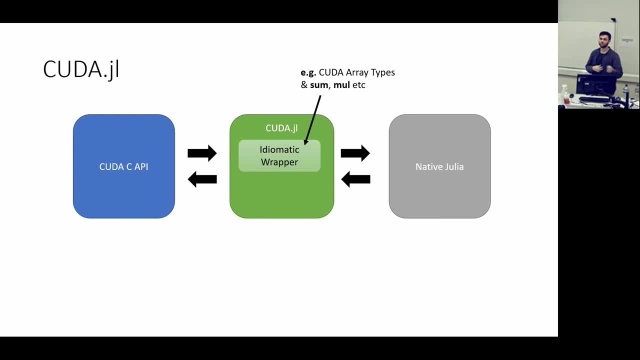 it a CUDA array. it will use the CUDA version of the sum function or the reduction there, and it's the same for, like broadcasting, mapping, sign, matrix, multiply. it will just point it to the right place in the CUDA library for you. We'll see what happens next. 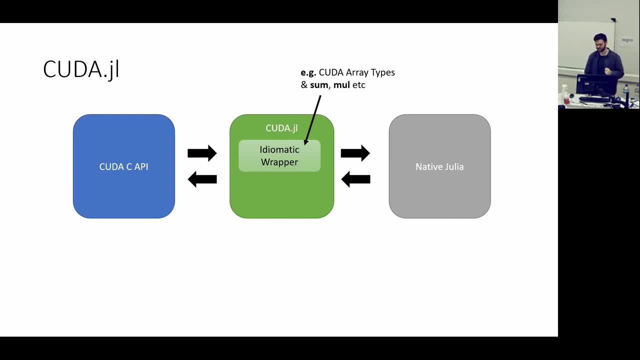 Thank you. We'll do this in a lot more detail in a few minutes. so something that's also quite special about this, which is quite different from other languages like Python, for example, is like: Julia is compiled- it's just in time compiled- so that means that you can essentially write some bindings to directly. 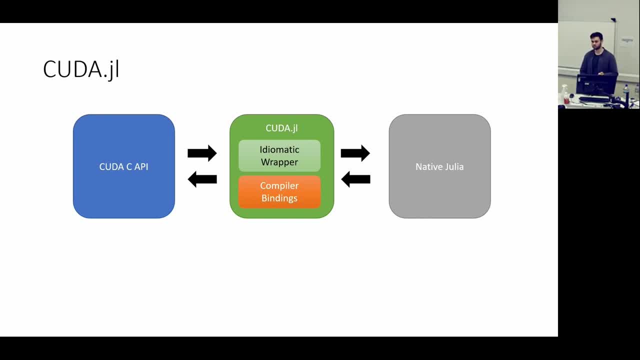 generate your GPU machine code for you from the native Julia code. so we're not restricted to only using what's in the C API And having to write our kernels in C. we can just write what we need in native Julia. so, again, Julia's compiler is called LLVM, and LLVM is like a way of making, a way of allowing you to compile code to a. 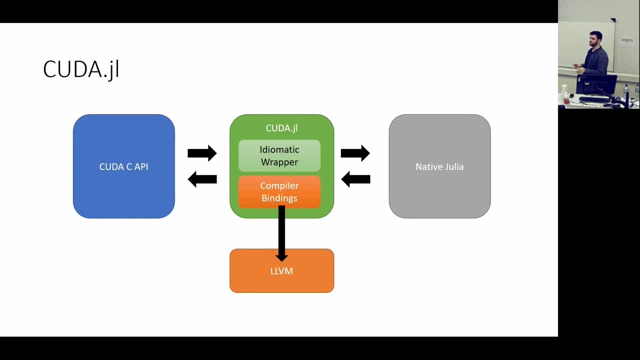 lot of different back ends, a lot of different devices, including GPUs. so essentially what happens is you can write some native code in Julia, Use CUDAjl's sort of compiler bindings, which then uses LLVM. LLVM then creates your device code to run your essentially your native Julia code directly on the. 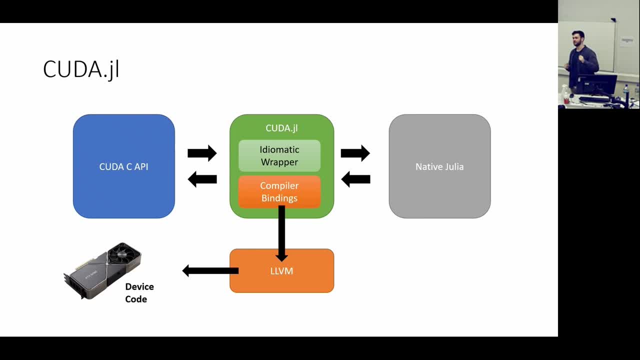 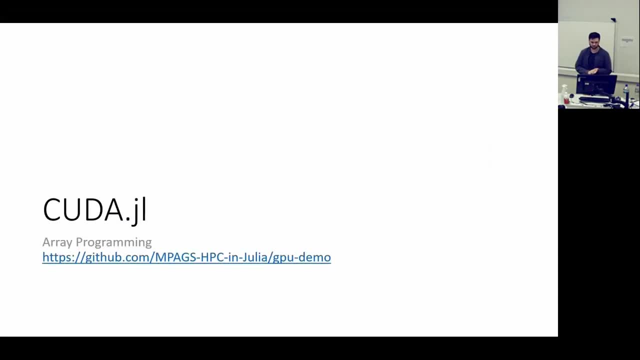 GPU without having to cross into another language at any point. Again, we'll see this in in just a minute, So for the rest of this we'll go over sort of a demonstration. there is a github repository with all of the examples that we'll go through. if you want to look at this. 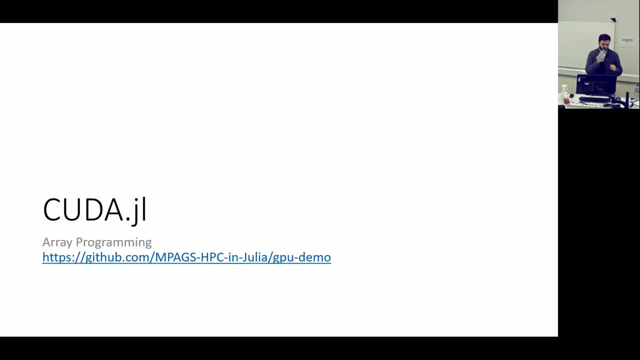 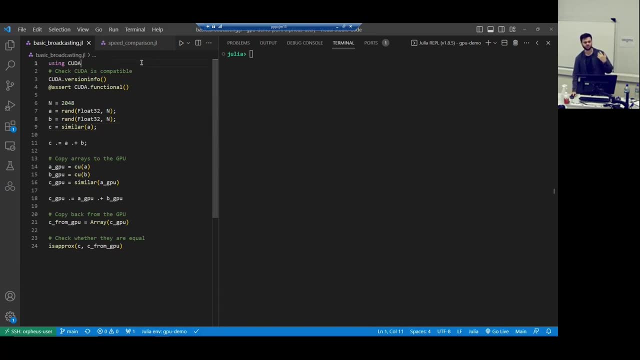 now or after the lecture as well. Okay, we'll go through how we'd actually use CUDA. So the very simplest, easiest way of using CUDA is to just change your arrays into the CUDA array equivalent type and write your Julia code using, like, your broadcasting notation. so when you 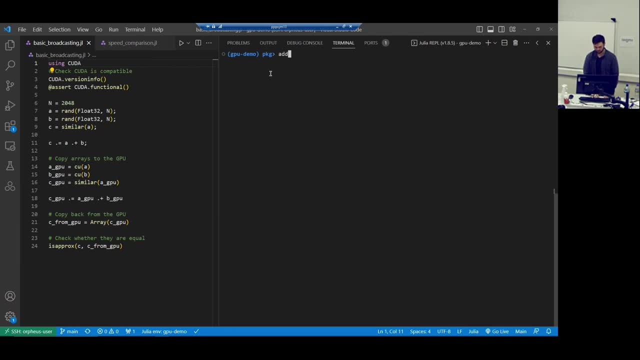 actually add CUDA. so if you're in the Julia ref or you type add CUDA, it will download the package for you. and also, if you say using CUDA, if you don't have the CUDA libraries installed, it will download them for you at this point and install them, which is quite nice. you shouldn't have to. 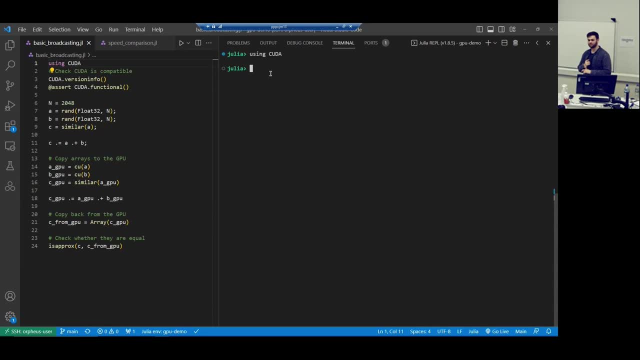 leave Julia at any point. to install anything else, you will need an NVIDIA graphics card and also the NVIDIA drivers installed. but if you have it in your computer, you'll likely already have the drivers. So this command checks the version info and it basically tells you what versions of all of the 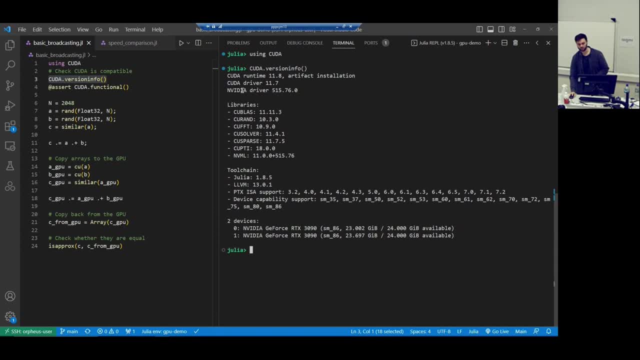 internal libraries that you have and also which graphics cards you have available. So usually you'll see one device at the bottom and it will tell you which device that is, which is good. if you don't see any devices here, that's probably a problem. you need to find a computer with one of these devices On the website. actually, there's a. 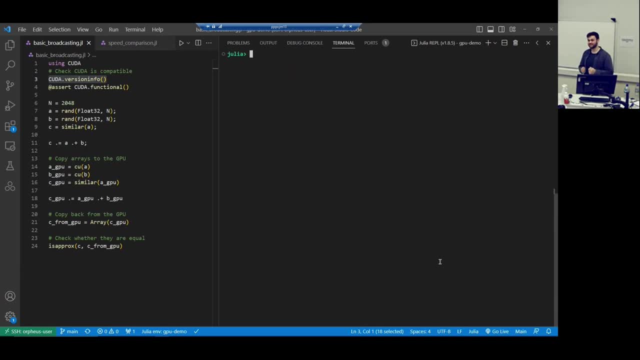 link to a Jupyter notebook which, at least as of a month ago, allowed you to spin up like a Jupyter notebook on Google Colab with a GPU enabled, and you can use Julia with it as well, if you want to experiment. You also want to check whether CUDA is actually functional or not. you only have to do this. 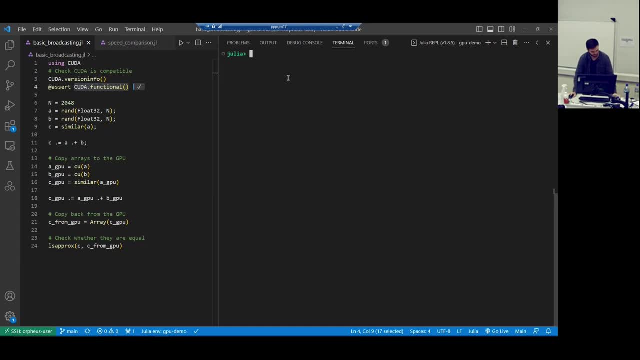 like once on one machine, just to make sure everything's working the way you expect. So hopefully this code will be very familiar. all we're doing is creating three arrays- a, b and c, which are just vectors. a and b are just random numbers and c is just allocating some memory. 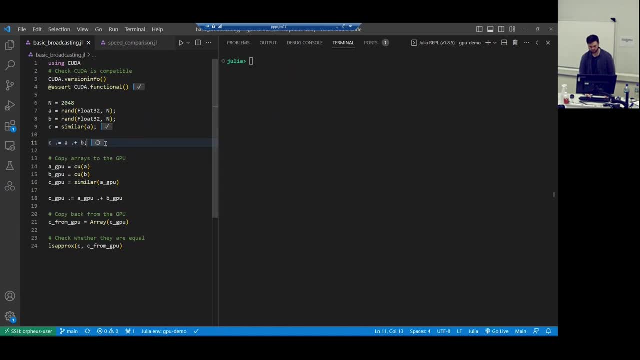 using the similar function and you'll note that we can use this broadcasting notation. so c- dot equals b to do element-wise addition and the dot equals means that we're storing the results of the element-wise addition into the array c on the left-hand side. So the way this works on the GPU. 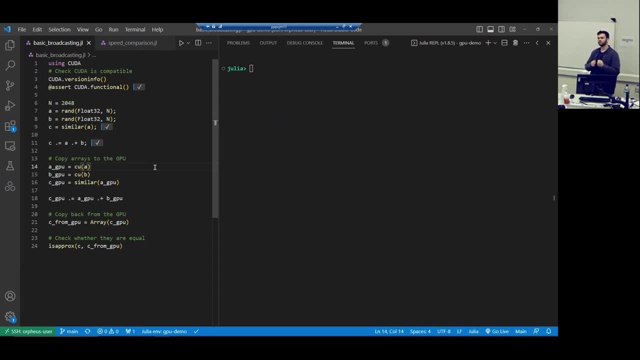 is well, for starters, the GPU can only access memory that's on the GPU itself, and currently these arrays are just on the host device. so we call the host, like your main memory, the main computer, um, and so we need to. before we can do any computations at all on the GPU, we need to copy the memory from 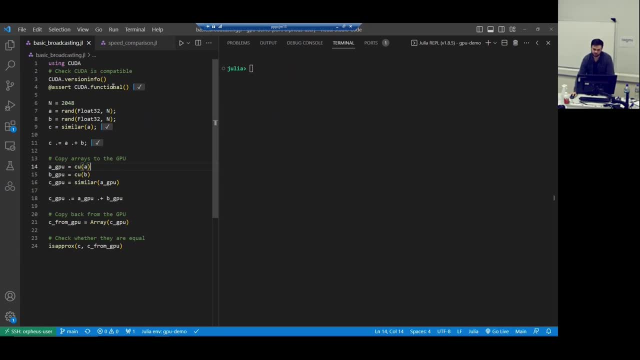 the host memory, the CPU, onto the device itself. so CUDA provides this function, cu, which basically converts an input array into a CUDA array. so if we, if we run this command, you can see that now right. so previously a was a vector of float32s, or a one-dimensional array of. 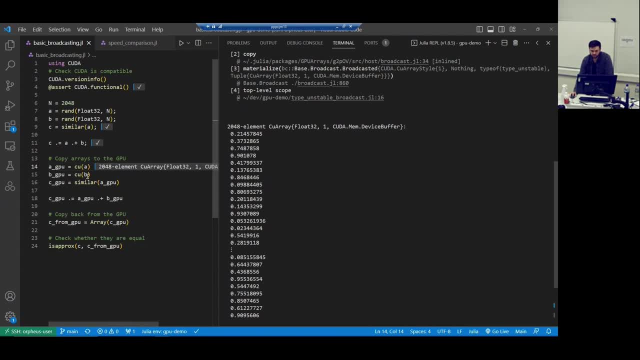 float32 values on the CPU. now, when we use a cu function, what we do is we copy over that array onto the GPU itself, and the array type has changed. now, instead of a normal array, it's a cu array or a CUDA array. we can do the same for b and now for c. we can use the same similar command, the exact same. 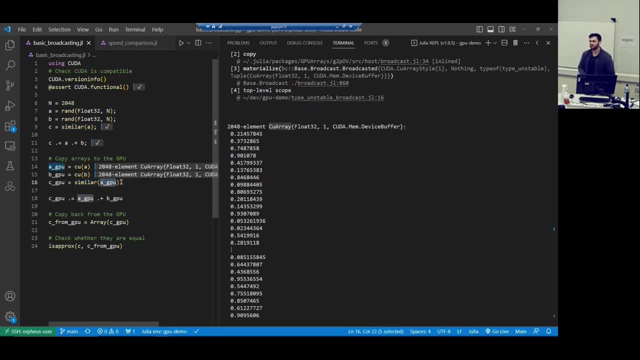 function. we don't have to call a different function and because the a GPU is of a different type, it will know um to create the similar array on the GPU itself. so again we run that and we get another CUDA array and we notice, or hopefully you can notice, that this line 11, this broadcasting, 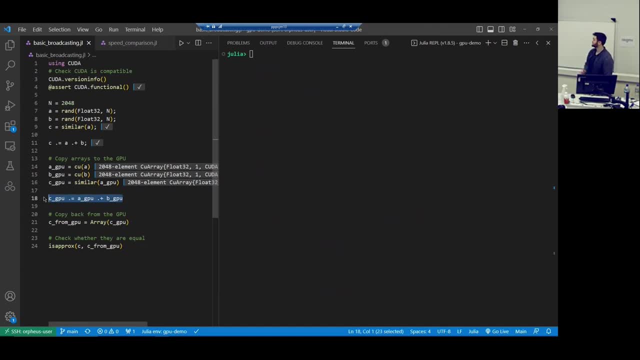 operation is exactly the same as this next operation on line 18.. um, the only difference is we're using the GPU versions of the arrays. we haven't changed any other source code. we run this. it works just fine. um, it compiles everything. uh, works great. so we just did a vector addition on the GPU. 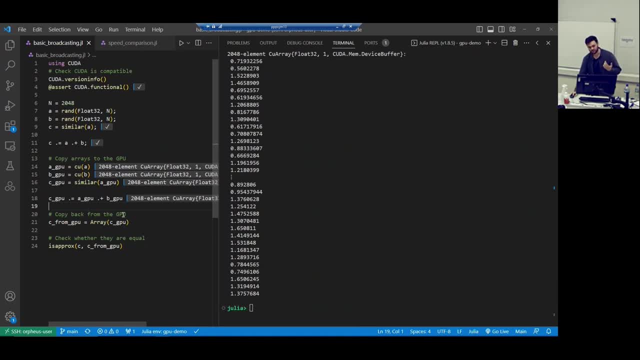 just by changing the input types to the source code. now we can actually check whether it works by comparing the results of the addition that we did on the CPU to the one that we did on the GPU. but to compare them we have to copy the results from the GPU back into host memory so we can. 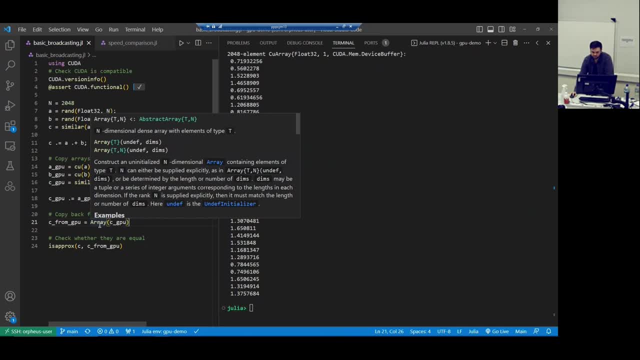 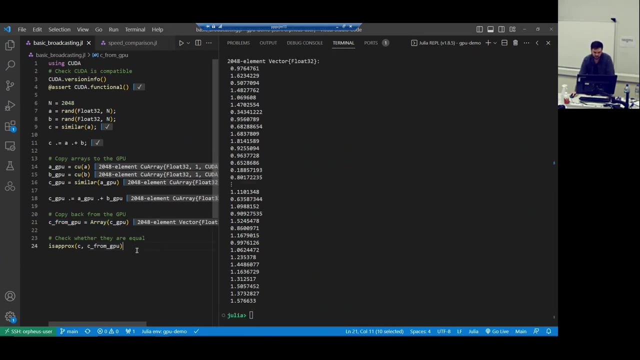 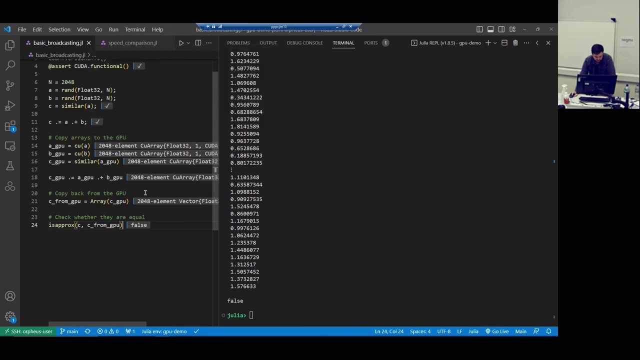 actually do the comparison. so, again, you can use this array um, basically convert it to an array by taking the c on the GPU and then putting it back into host memory. so this is just a copy and then you can use the is a prox function to check whether they're correct and you can see here it's actually wrong. 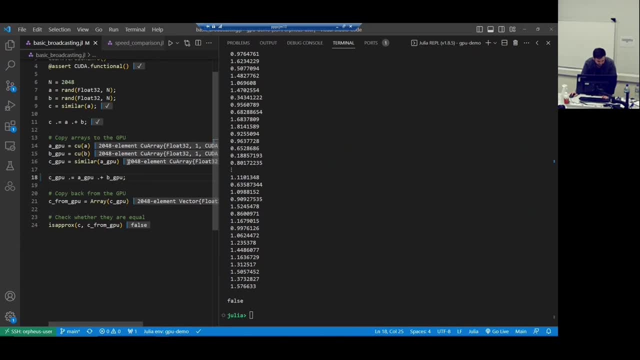 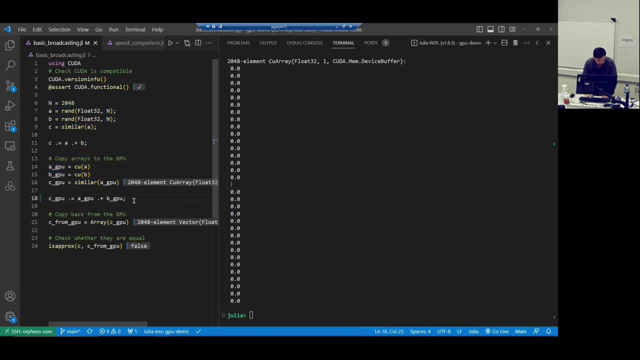 so let's work out why it's wrong by running um and copy back. okay, all right, rerunning everything. it worked, it was fine um. so yeah, this um basically means that you can offload safely to the GPU. we use this as a prox function because the floating 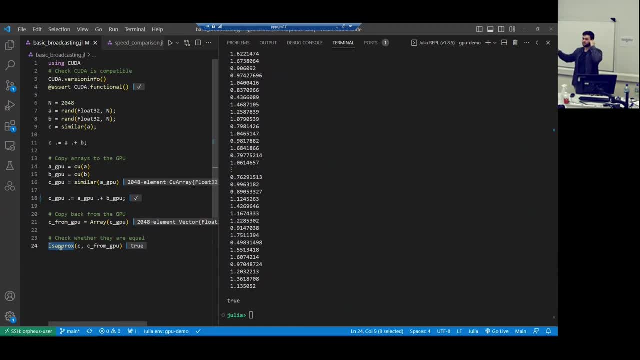 point, math might be a bit different to how it works on the GPU, to how it works on the CPU, so you might get very slightly different results, and so they probably won't be exactly equal, but they'll be approximately equal, okay. so, um, yeah, i'll do a quick speed comparison. I'll just run this first so we don't have 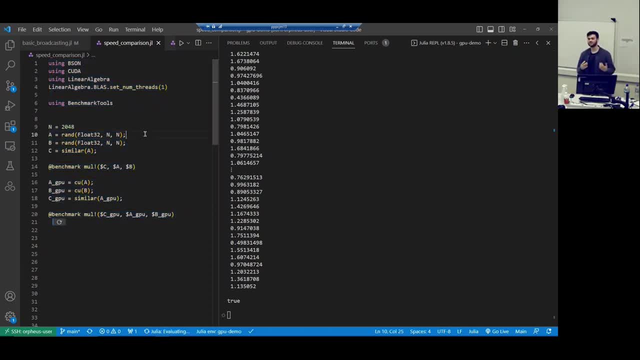 to wait for all of the results. but this is essentially the same example, but instead of doing a vector addition, we're just multiplying two matrices by each other and storing it in another matrix. so the linear algebra base library package provides this function, mole bang, which basically says: do like times A and B together. 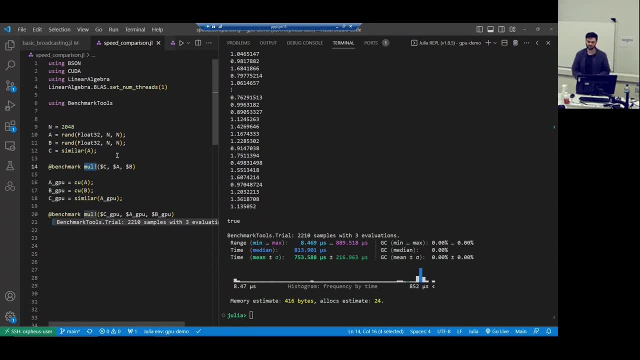 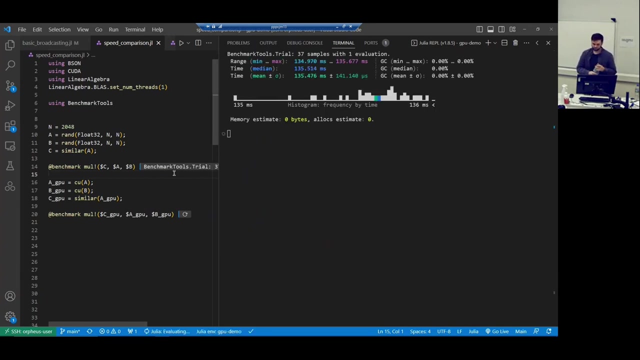 and store the result in C, where C comes first. Okay, so if we benchmark the first example and then the second example, we'll see one important factor that comes into when you're actually programming with a GPU. Okay, this might take a long time to benchmark, but we can see it takes. 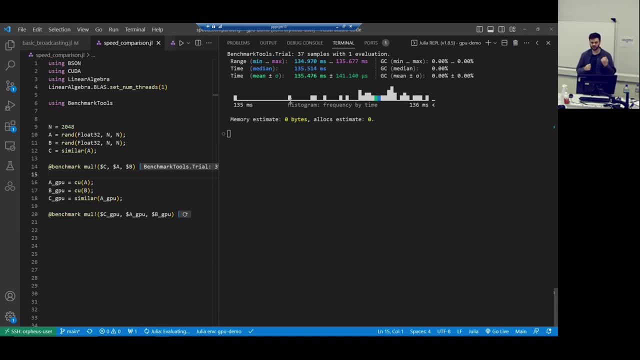 around 135 milliseconds on the CPU to do the matrix multiplication. We've made sure that we're only using one core as well, with this set number of threads at the top. But we can see on the GPU. well, for starters, this is a huge range. It goes from eight microseconds all the way up to 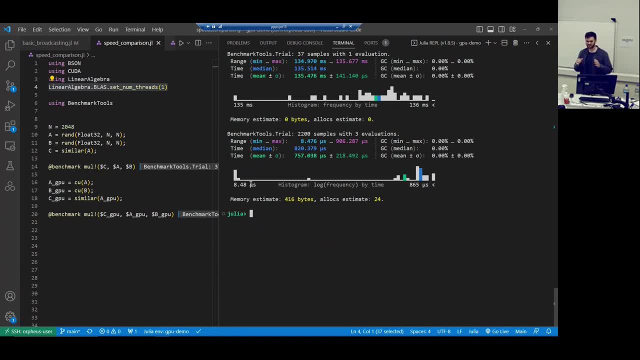 900 microseconds, which is quite a big difference, And the reason is we haven't done our benchmark correctly on purpose, but we haven't done it correctly So because the GPU is a separate device from the CPU. whenever you want to do work on the GPU, it doesn't make sense to make. 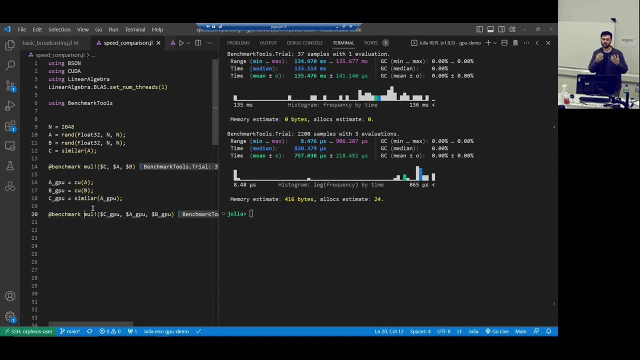 the CPU just wait around for the results. So whenever you launch work on a GPU, the CPU will just continue processing. So it's kind of like this ACM. So if you've done the parallel programming workshop, it's like this: threads at spawn. 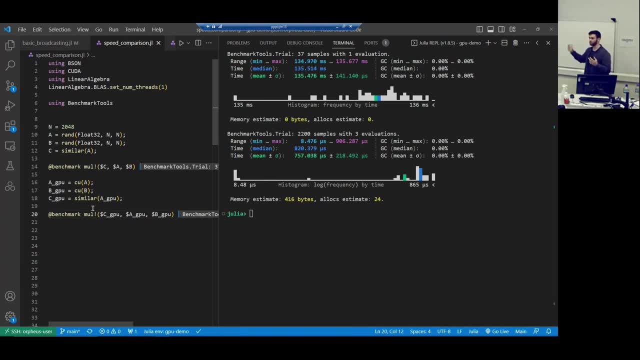 It will just start the work on another thread and then just continue with whatever's happening. So in order to time this properly, we have to use this cudaatsync macro to make sure that any work that was launched on the right-hand side of the macro is completed before you exit. 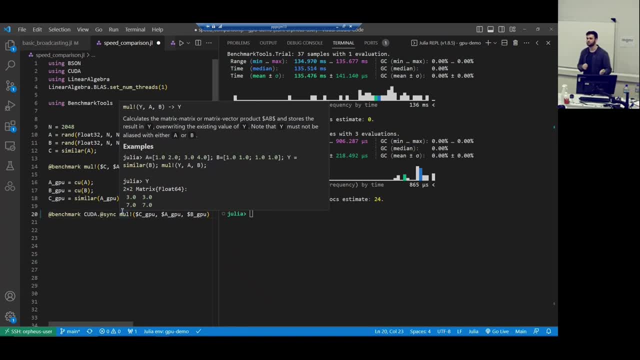 So this is just like the synchronization or fetching. So this is the fetching step that you would do in your sort of normal asynchronous programming. So when you set these numbers for s equals one, is it on the CPU or on the GPU? Sorry, which line? 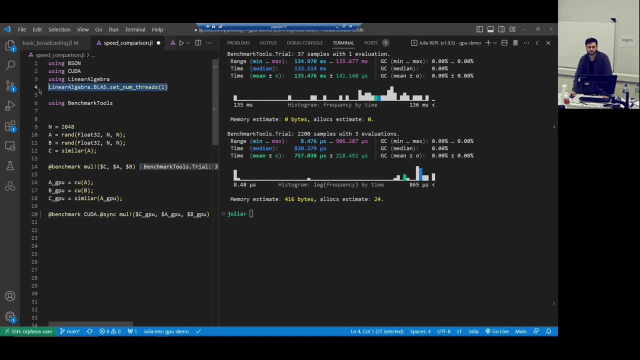 So at the beginning you set the numbers for s equals one. Yeah, this is just for the CPU. Just for the CPU. I said that this small bang function comes from the linear algebra library, but cuda implements an extension, So that which works with cuda arrays, which calls the underlying like blast library defined in cuda itself. 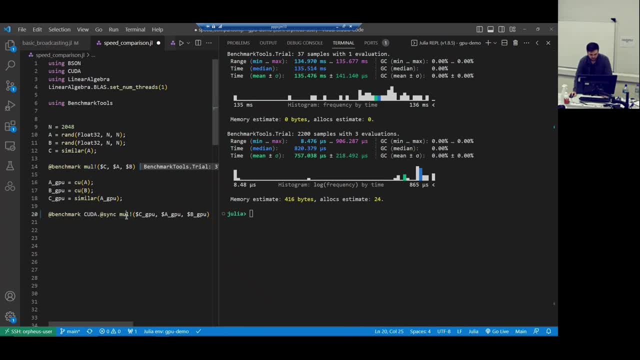 So yeah, if we rerun the benchmark with the atsync macro, we should see benchmark timing. that makes a lot more sense. So yeah, if you're ever benchmarking some GPU code and it takes far less time than you're expecting, it's probably because all you're doing is timing it. 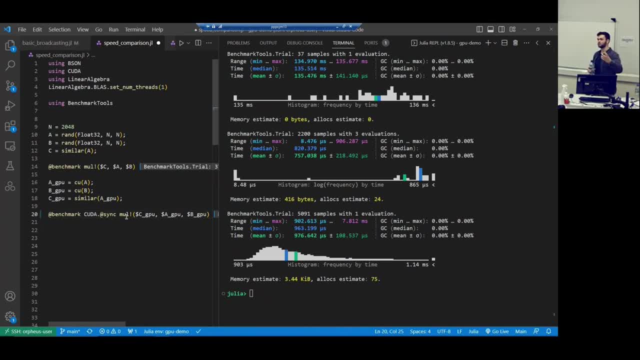 Timing is timing how long it takes to actually schedule the work on the GPU, not how long it takes to actually execute that work. So yeah, so you can see this is much more sensible. It's between 900 microseconds to about 1.1 millisecond. 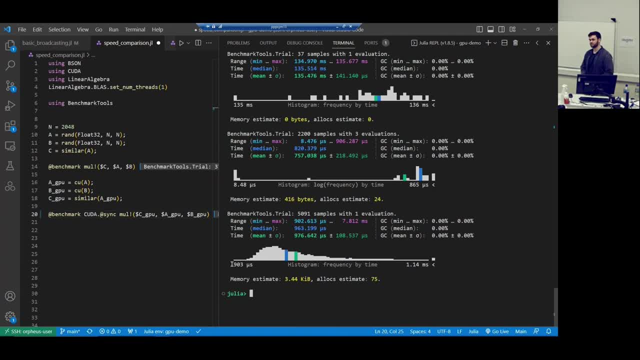 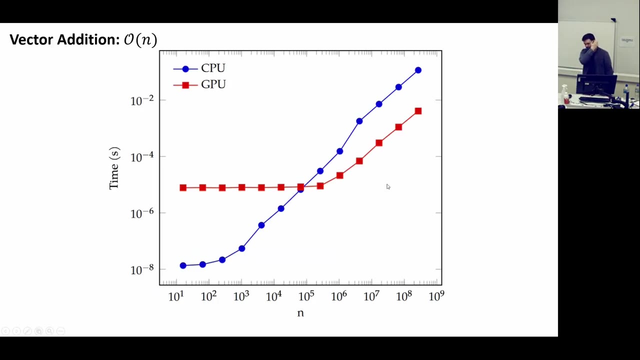 And you should see this is about 130 times faster than the CPU. So GPUs are really good at this sort of parallel processing, especially with big arrays. So if I just quickly switch back to PowerPoint, So this graph just shows the timing, So the actual timing like in seconds of running just an element. wise vector addition. 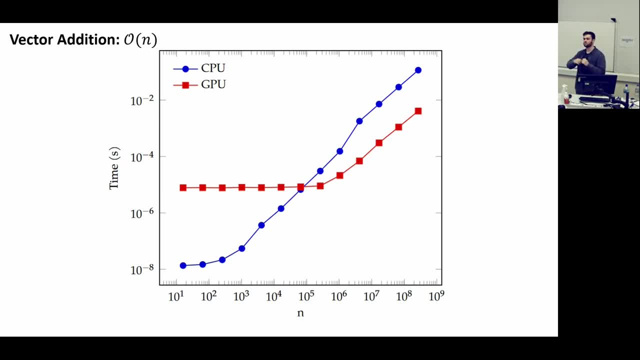 like we showed in the first example. But we change the number of elements with n on the x-axis And you can see this flat line for the GPU until we hit around between 100,000 and a millisecond. This flat line is the time it takes to actually schedule the work on a thread. 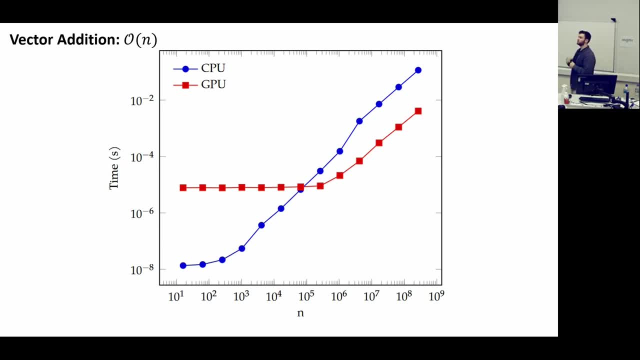 So you're paying this cost every time- It's like the overhead just for launching this kernel. So for most examples it only really makes sense to do work on the GPU if you have enough work to give to the GPU to overcome this cost it takes to actually schedule. 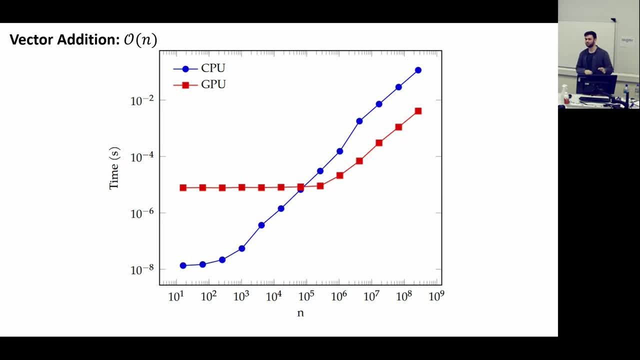 the work there And this cost is about- I mean, we saw it before it said about 8 to 10,000.. 10 microseconds, It'll depend on your machine, but in that sort of range. So you want it to be doing at least that much work just to sort of compensate for the overhead. 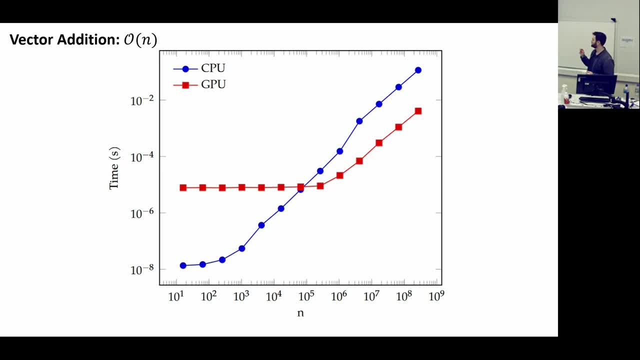 What it also means is you can scale up to a huge number without incurring any additional cost. So, for example, it takes the exact same amount of time to do a thousand elements as it does to do 10,000 elements. in this example, 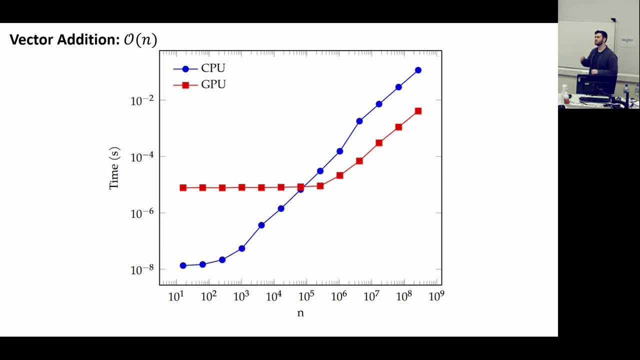 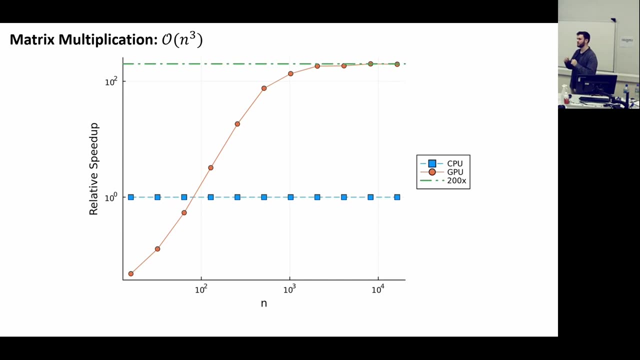 So it's quite nice. You can go up to higher sizes for practically no cost if the array sizes are still quite small. As another example, if we go to matrix multiplication, which is order n cubed instead, we hit this threshold at which the GPU becomes faster than the CPU a lot earlier for a lot. 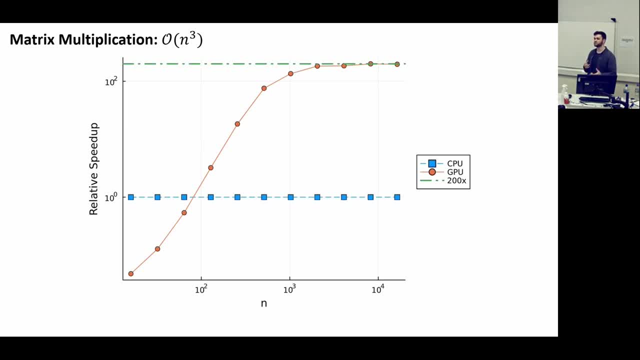 smaller matrix sizes because matrix multiplications are much bigger operations. You're doing more computation. So here we. as soon as we're hitting around a hundred elements, like a hundred by a hundred matrices, the GPU becomes a lot better. And by the time we get to like 10,000 by 10,000 matrices, the GPU at least on this machine. 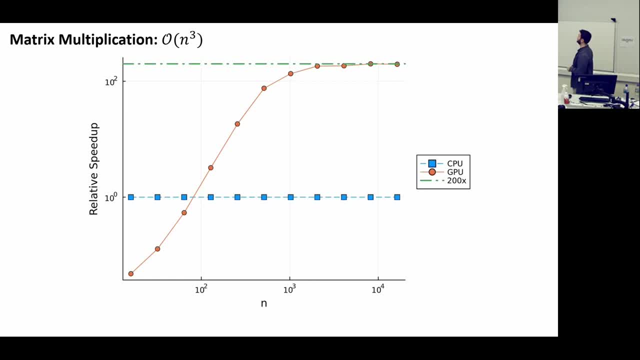 is about 200 times faster than the CPU. It will saturate when the GPU sort of runs out of more cores to process, to process the matrix. So yeah, GPUs can be very fast as long as you give it enough work to do at a time. 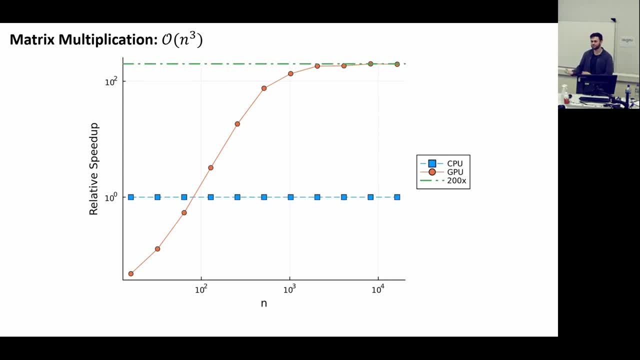 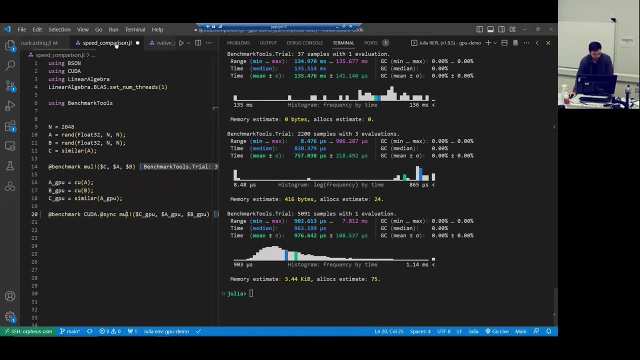 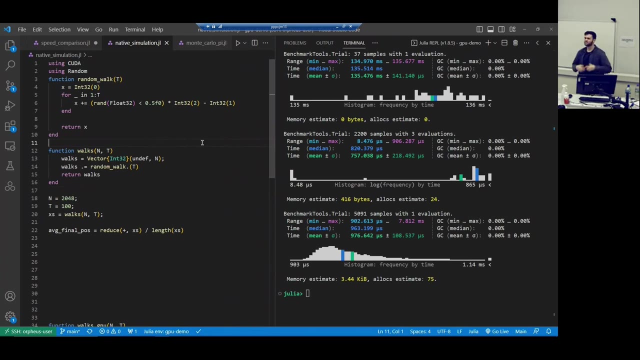 But there are a few extra things that you can do. You don't just have to do like vector addition and matrix multiplication, And we'll take a quick look at those. So remember before I showed in one of the previous lectures a random walk. 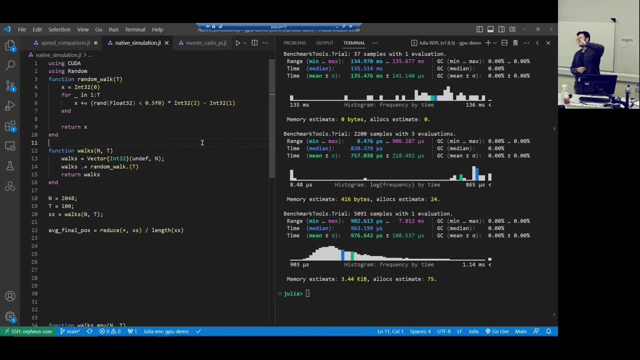 So you just have a point in there. So you just have a point in there. So maybe now you get it in space and you randomly move in some direction. The specifics aren't important. What is important is we can define a function in Julia to perform this that will work on the CPU. 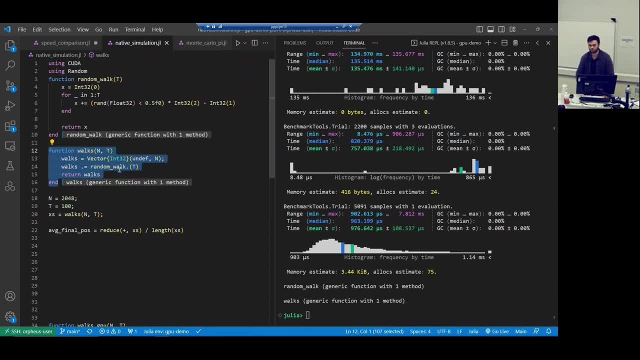 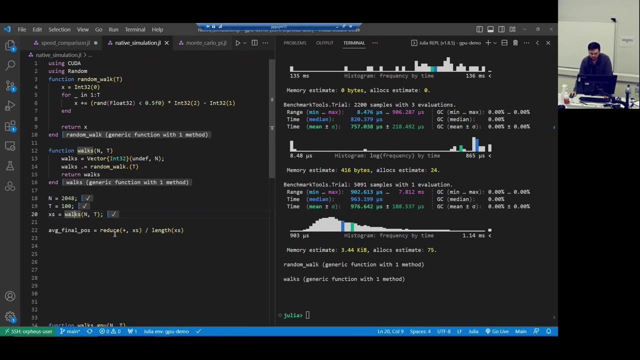 So this is your custom code itself, and you can write a function that will generate N number of these walks. Just perform it many times, And here I'm just using some broadcast notation. save me having to write a for loop, And so we can give some parameters and call this code. 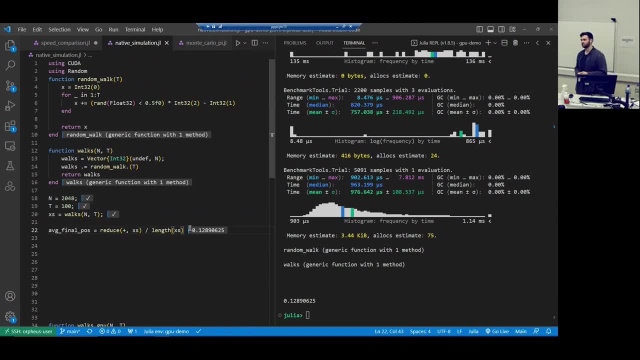 We can, for example, find out the average end position of one of these walks. Obviously, it depends on your application as to what you want to compute, but let's say we actually wanted to take this process and move it onto the GPU instead. 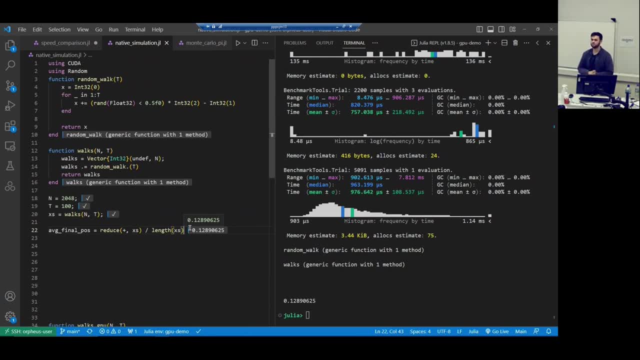 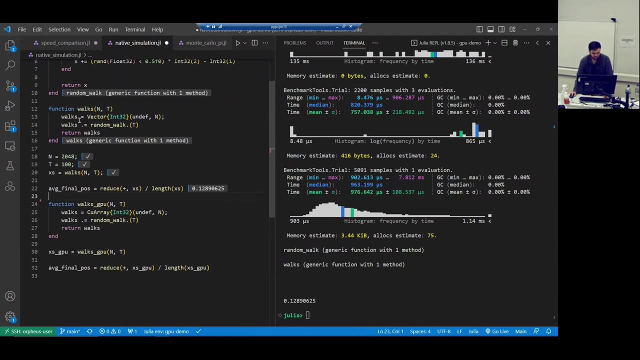 So instead of having to completely rewrite our code to make use of the GPU, we only rewrite a little part of the code itself. So for the GPU version I will remove this space so we can compare. So in the CPU version we created an array to store all of the values of our walk. 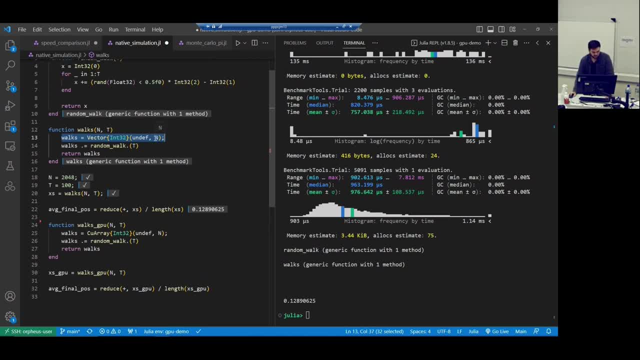 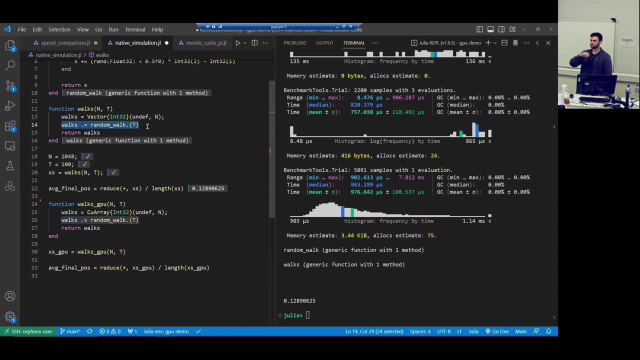 so the positions themselves? Yeah, so the positions themselves. And then we actually perform the walk, storing the results in this walks array. And here, instead of creating an array on the CPU, we just create an array on the GPU using the GPU array type. 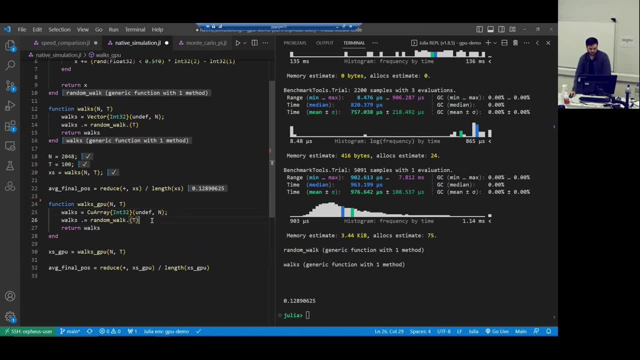 So these lines are the same, apart from the type. Nothing has changed. The next line is identical: is exactly the same code. The only thing that's changed is you're using a broadcast operation, but you're storing the results in a GPU array. 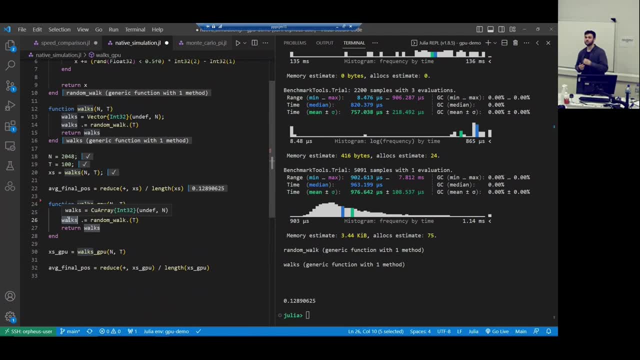 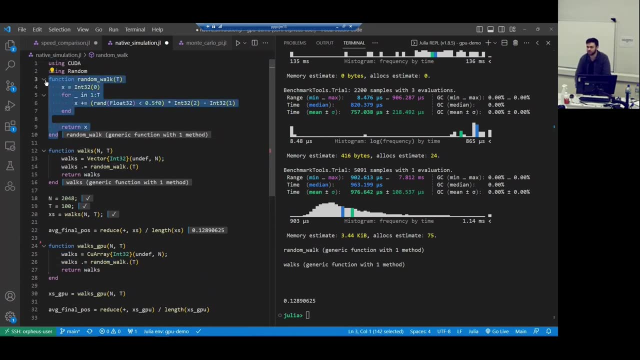 So this basically is the same code. So this basically is the same code. It just basically tells the compiler to use the GPU code to execute it instead of the CPU code. This random walk function is the same function that we specified in our native, pure Julia code. 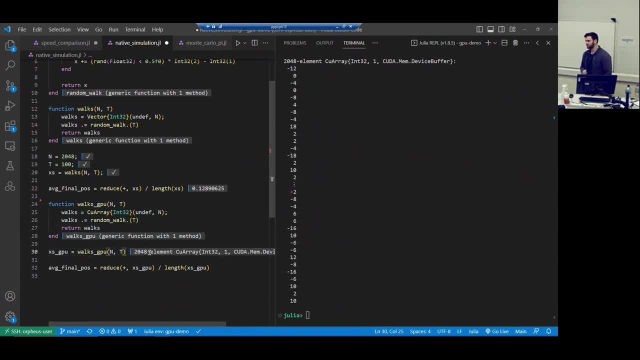 So if we define this function and run it, it might take a while to compute the first time, but it runs perfectly. So we didn't change the vast majority of our simulation. We just changed some of the types and it was able to run. 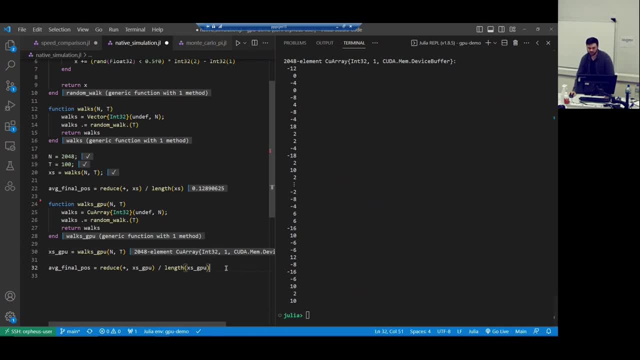 And it was able to compile it and run it on the GPU. And again, CUDAjl gives implementations for reductions as well, So you can write your own reduction. You can write your own reduction to sort of use all your code very generically. 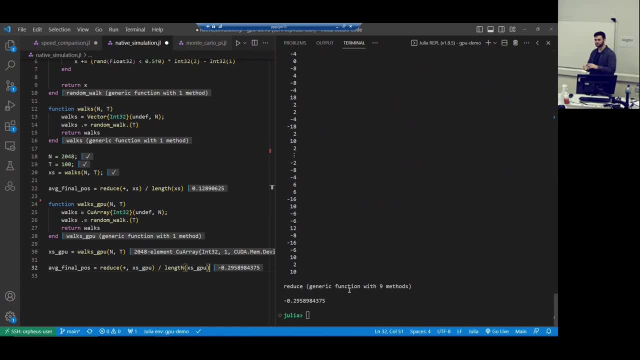 So if you write your functions with broadcasts, reductions, maps, the very sort of general generic versions, perhaps all you have to do is change the types and your code will probably work on a GPU. So this is your sort of your first port of call. 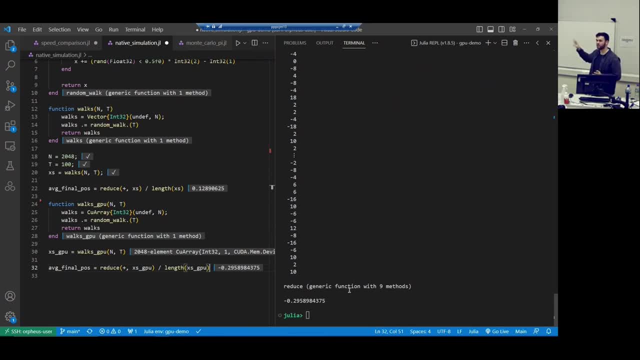 when you want to get something running on the GPU right in this sort of generic vectorized NumPy-like form And you should be able to quite easily transfer to a GPU. Won't work for everything, which is why we have another session on Thursday. 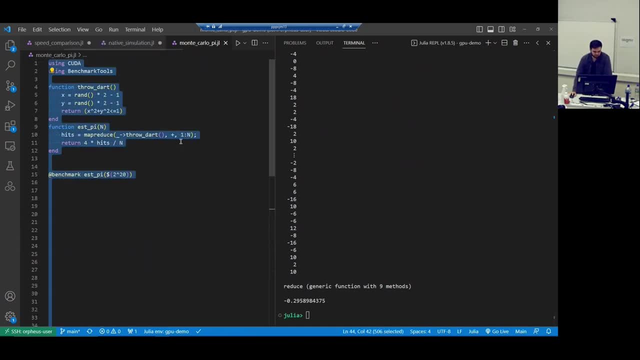 to go over the case at the edge cases, So I will very quickly go over this example. So in the previous lectures we talked about estimating pi by throwing dots on a dot board and measuring or counting the number of dots that hit inside a circle. 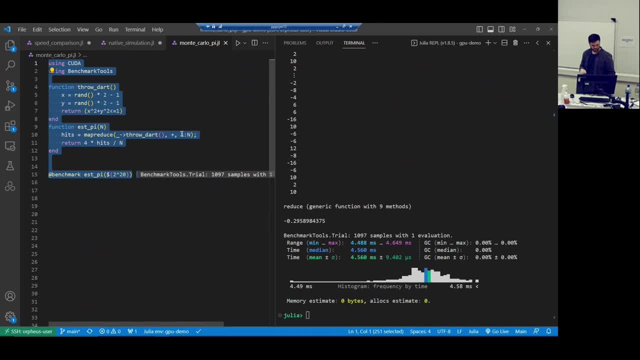 as opposed to sort of outside in the square regions. So yeah, just in case some people missed it. So you have a circle whose edges just touch a unit square. you have a unit circle and put a square just on the outside and you randomly throw dots inside. 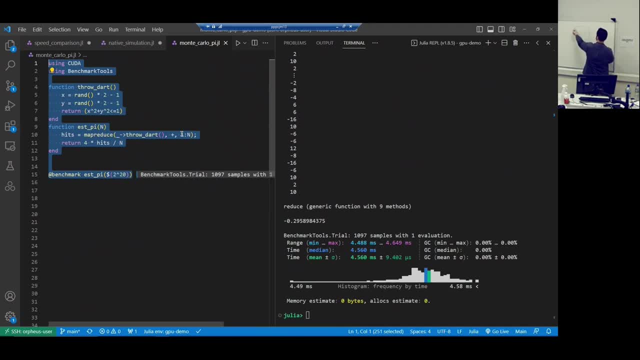 and you count how many land inside the circle as opposed to landing outside And the sort of ratios of this you can estimate pi, Yeah, So this is some very reduced code to do that on the CPU. just one call And again our function for actually throwing the dot. 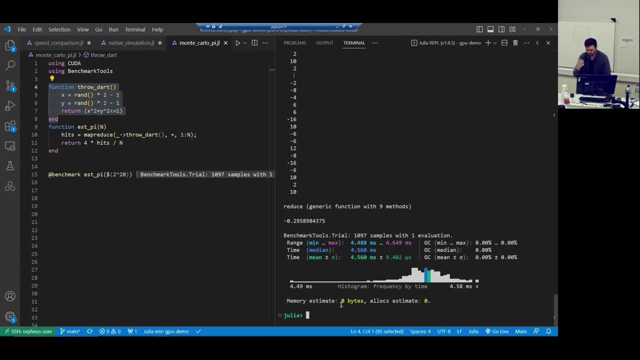 is just written in pure Julia And you can see. this takes maybe around four and a half milliseconds when we benchmark it. When we go to the GPU again, I'll get rid of this side. So this was our CPU implementation and this is our GPU implementation. 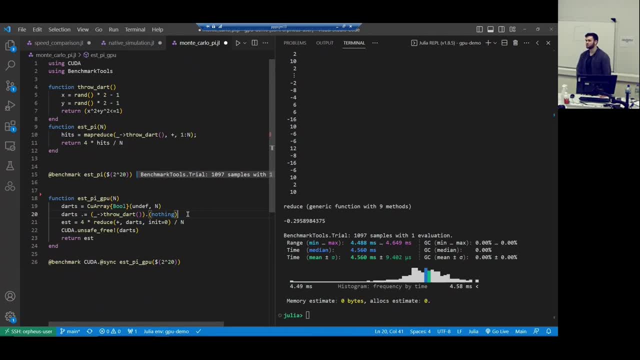 Here we can't quite do the same thing just using the generic functions. So instead what we've done is just created an array to store whether a dot is hit or not. So just a ball yes or no, And we calculate that first. 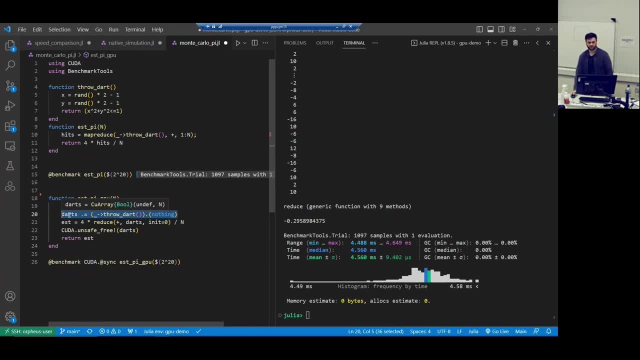 So we throw all the dots. we'll get a series of zeros and ones back in an array, And then we'll use the reduction function again to basically count how many hit and how many didn't hit. Anyone want to have a guess at what this line does? 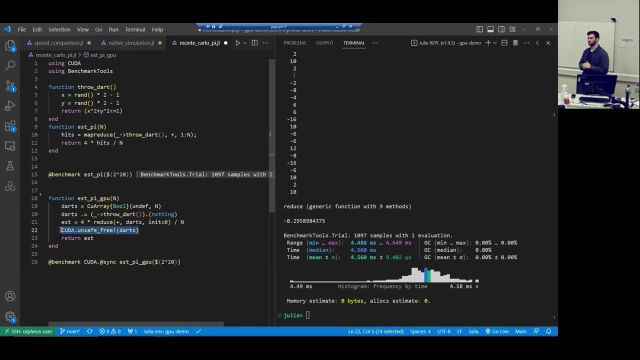 It's unsafe, free and you pass it in array. Anyone since C before this should look somewhat familiar. Nope, that's fine. So this first line: what we're doing is allocating an array on the GPU. So we say we want to. 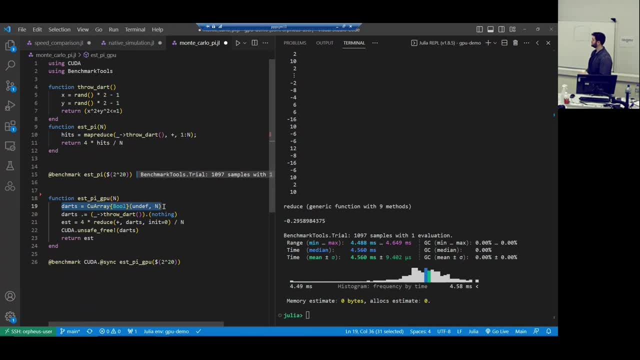 I'm just talking, but I said I remember No problem, no problem. So yeah, So we're allocating some array to store all of these zero and one values, But afterwards we're not actually using it. We're allocating it and never using it again afterwards. 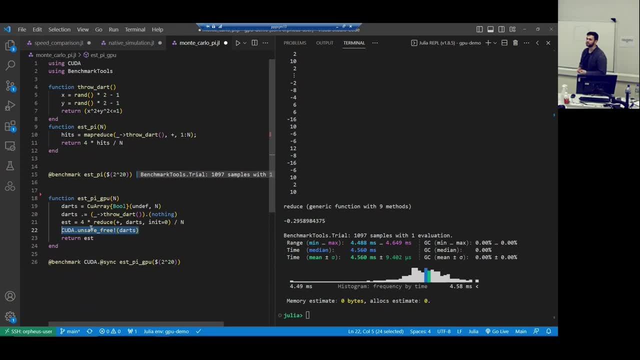 So CUDA provides this function unsafe free, which basically says we're not going to use this memory anymore. Feel free to use it for to allow it to be used for another purpose later on. It's called unsafe because if you are using that memory again afterwards. 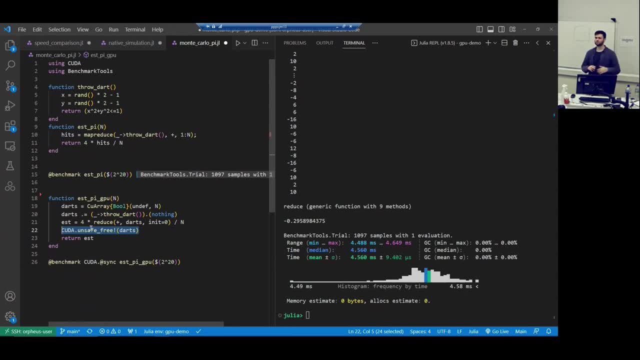 you'll get some memory corruption potentially. So when you're writing in C every time you allocate memory, you should also free the memory as well when you're not using it. In Julia we use a garbage collector and CUDA does implement some garbage collection for CUDA. 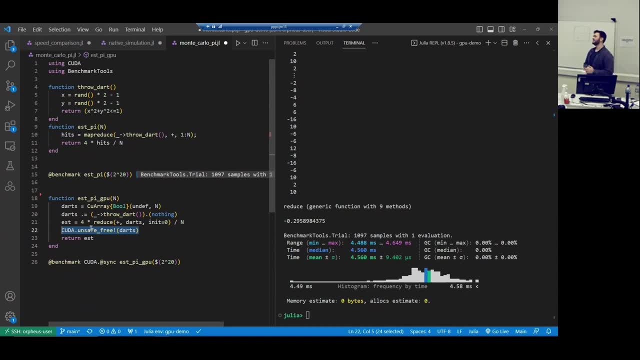 but it's not very good And it doesn't always work, And so this gives you a bit more freedom as to when you are going to use memory and not going to use memory, So it avoids some GC pressure, which can also help performance as well. 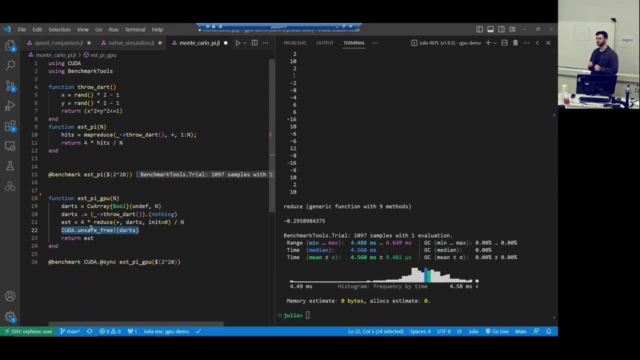 I should also mention at this point is GPU memory is usually a lot less than main memory, So most consumer GPU cards nowadays would have between like four and 12 gigabytes of RAM, Whereas it's pretty easy to find a computer nowadays with 32 to 256 gigabytes of RAM. 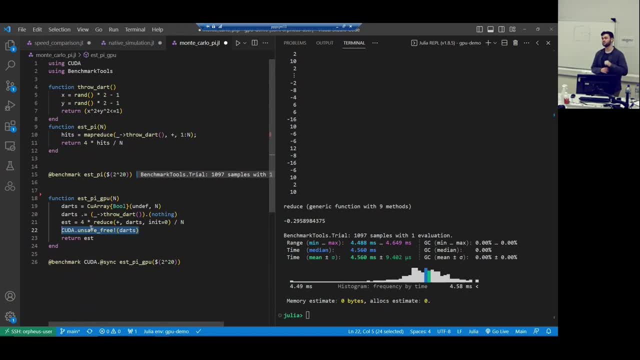 So RAM is much more of a precious resource on a GPU than it is on a CPU. So you shouldn't be careful about what you're allocating or what you're not allocating. So I bring up this example as a way that you have to sort of bend your algorithm a little bit. 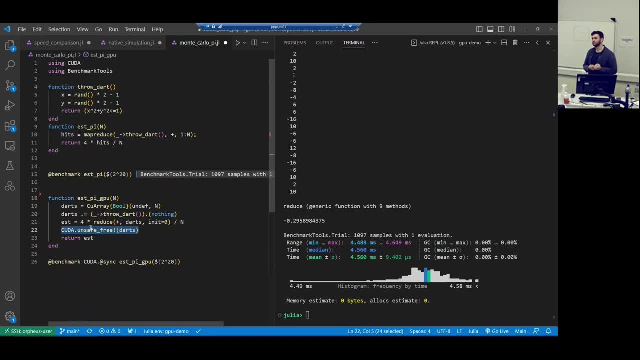 to work with this sort of generic GPU interface. So here we didn't have to allocate any memory at all, Whereas here we had to allocate some memory and then do another calculation on that memory. If we're writing our own kernels, we can avoid this. 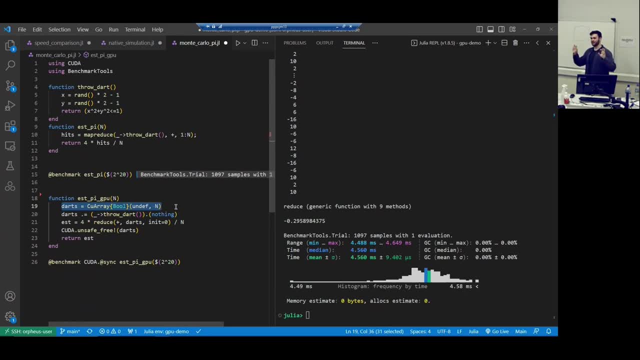 And so we'll talk about that next week. Again, a kernel is just a program that runs on the GPU. There's nothing special to the name at all. That's just the language that they use to talk about it, And so when we're actually 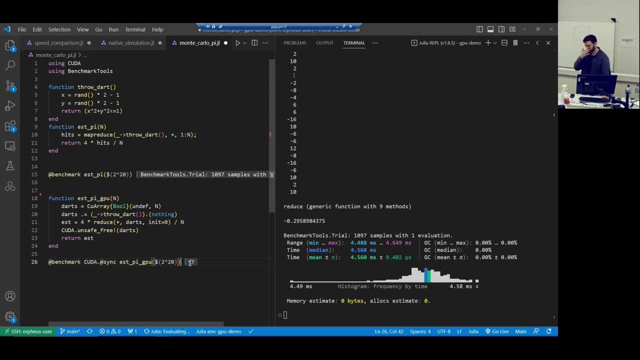 yeah, I should also benchmark this code. So when you're running some program that runs on the GPU, we say: you'll launch it, You'll launch a kernel, And so that will take some time, And so launching a kernel has some overhead. 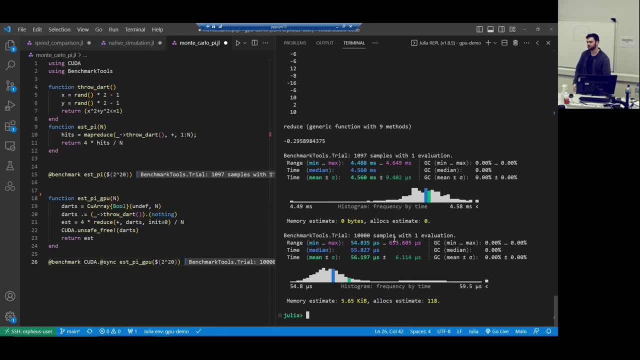 But you can see, in this case, even though we're allocating a huge array on the GPU, the GPU is just so much faster at this parallel processing that we get a huge speed up. So we went from what was it? 4,500 microseconds down to 54, 55 microseconds. 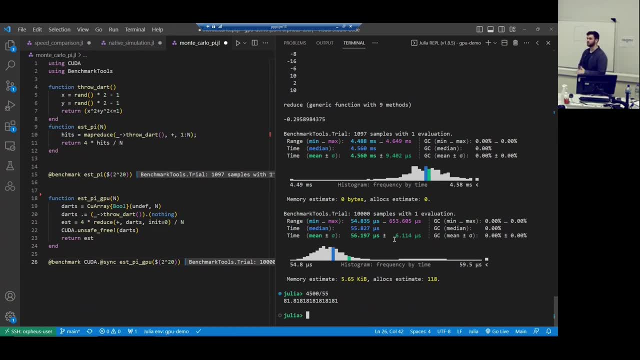 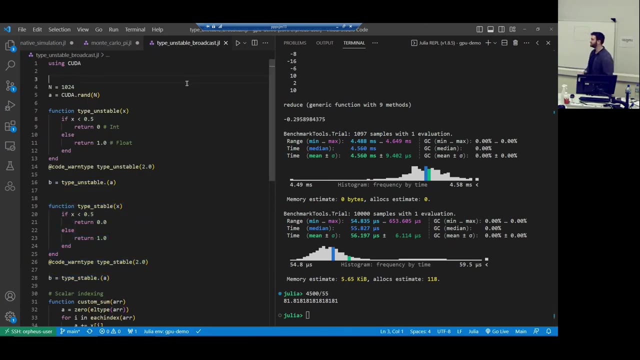 So there's about an 80, 80 times speed up, even though we're allocating this big array for this example. So allocation sometimes isn't bad if it gives you your results correctly, and it's good enough in this case. So this is all well and good. 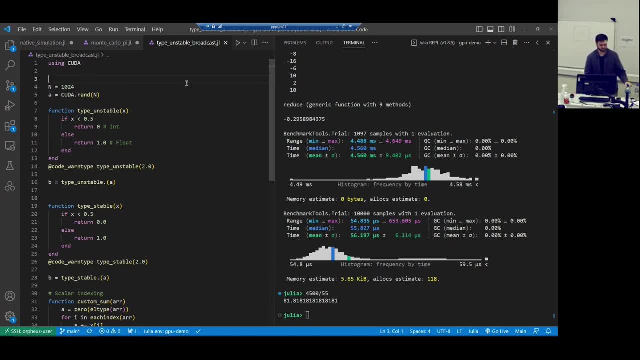 but there are some restrictions in how you write your code. So when we spoke about optimization in the past, we spoke about type safety is very important. Type safety and why it's very important in Julia. So type safety is just: the compiler knows what type everything is. 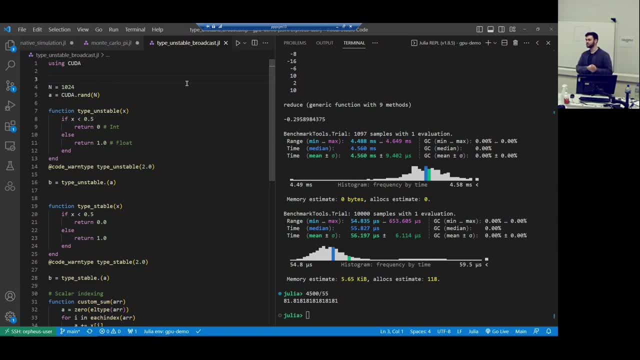 And so usually in Julia we don't say what the specific types of things are. We let the compiler work it out. but there are ways in which we can program to be careful, to make sure that it's predictable. So here's an example of a function. 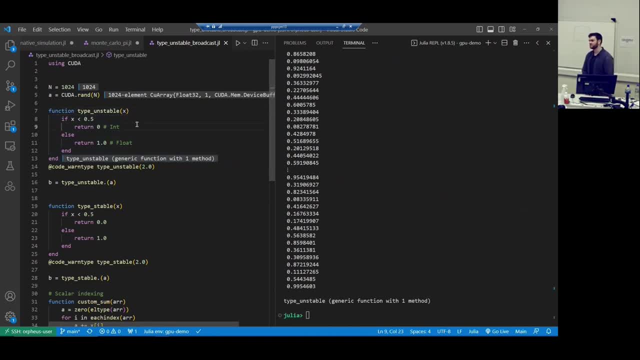 that sort of returns, two different values, And this is really easy to do, just saying like zero or like 1.0, or maybe it's like 1.5 or something, But what we're actually saying is depending on some runtime value of X. 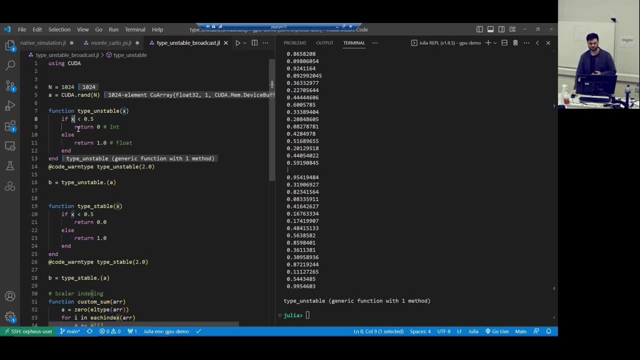 because the compiler doesn't know what value is stored within X when it compiles. it just knows, potentially, that it's a float or an integer or something along those lines: either return an int or a float, because we've written 1.0 instead of just one. 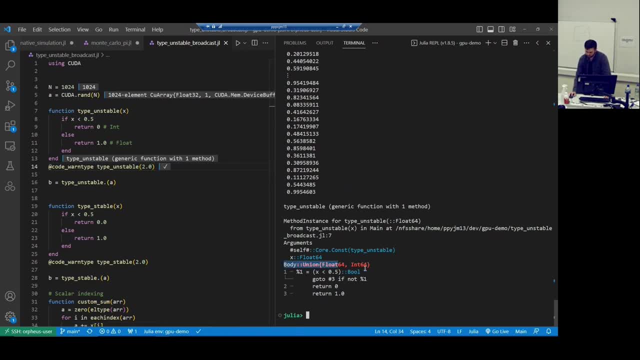 So if we use the code one type macro, usually you can see if something is type safe if there is a big sort of red highlighted section that says union of, in this case, float 64 or int 64.. So this is basically saying that this function. 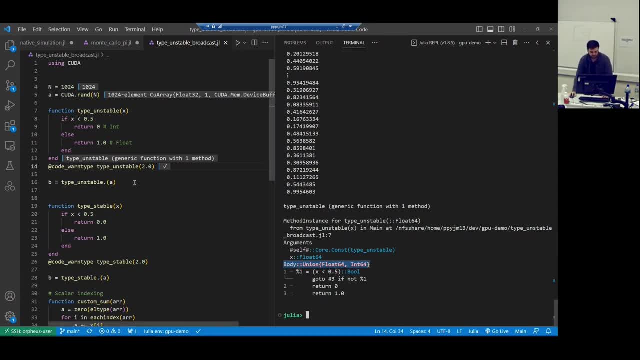 will return one of those types of values. And if we have created a GPU array and what we want to do is basically perform a map, So we map, using this type and stable function, each element of this A into another matrix B. 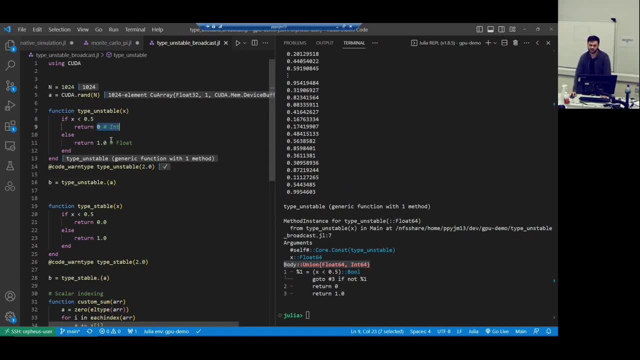 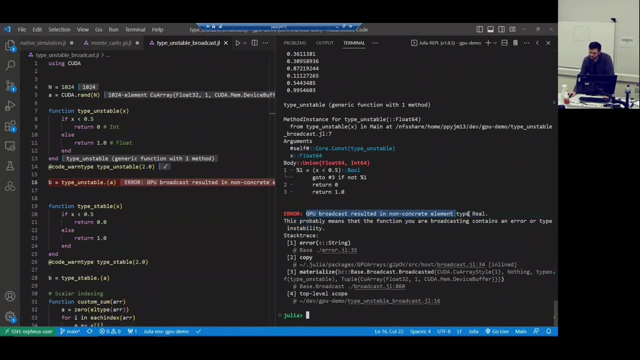 So this would be sorry. matrix a, vector B, which would have values of either zero or one. If we actually run this, we get an error, And the error that comes out says that the broadcast resulted in non-concrete element type real. 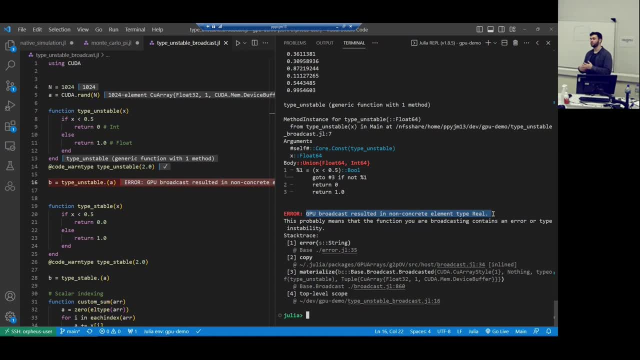 So that basically says it couldn't infer what the return type was And specifically it wants a concrete return type. So this is something that's at the bottom of the inheritance hierarchy or the type hierarchy in Julia. So these are your ints, your floats, your balls. 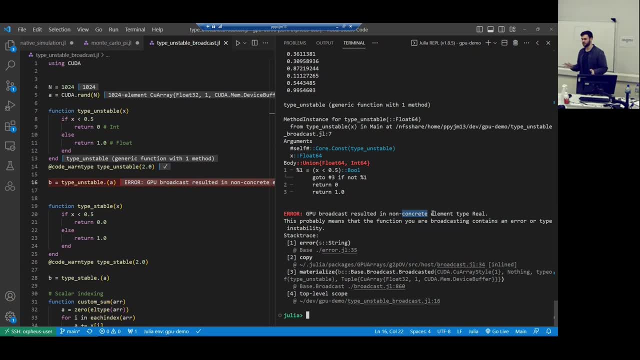 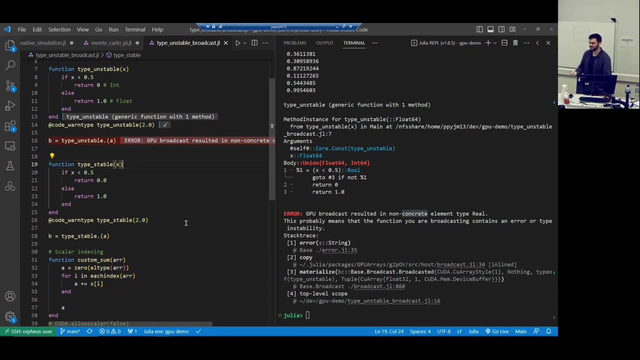 not like real values or numbers, which is an abstract type. So the way we fix this is again- you should do this for optimization purposes anyway- is just make sure your code is type safe. So if we change this to instead only return floats, 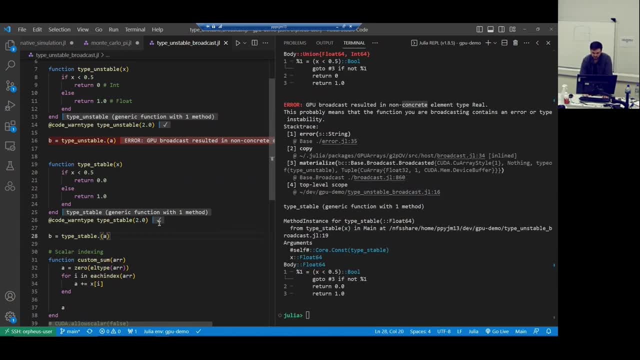 so either 0.0 or 1.0, we can see it's now type safe. The compiler can infer that you're getting a float out of this and then you can use it on the GPU just fine, And everything works exactly the way you expect. 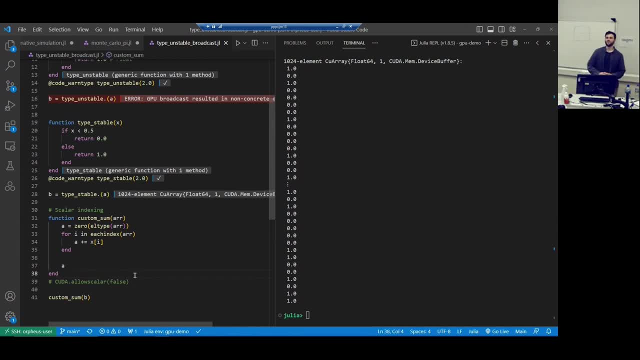 There is one sort of final thing that you will run into a lot in your code. At the start I said to you that writing your code in broadcast vectorized notation and writing it in a full loop makes no difference. in Julia, That's only true for the CPU. 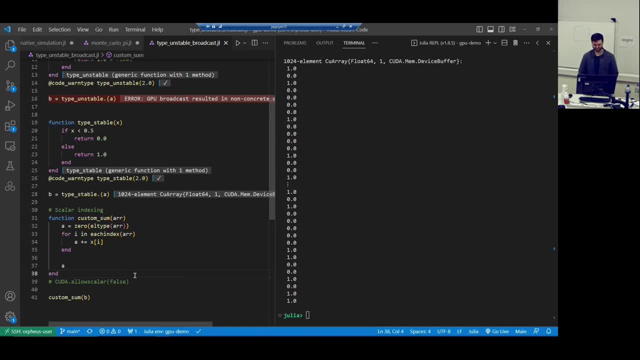 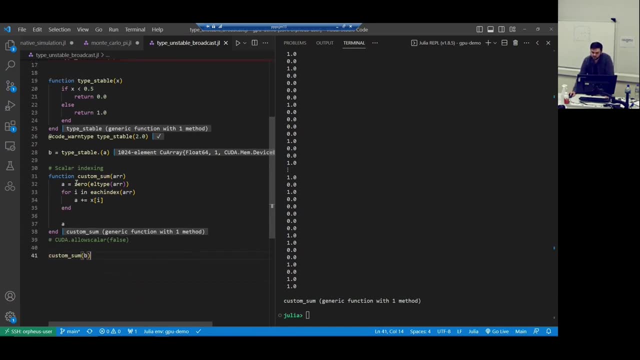 On the GPU. it won't let you do that. So if I sort of run this function or create this function which just tries to sum up all of the elements in an array, and I pass into it a GPU array- sorry, if I pass into it a GPU array- 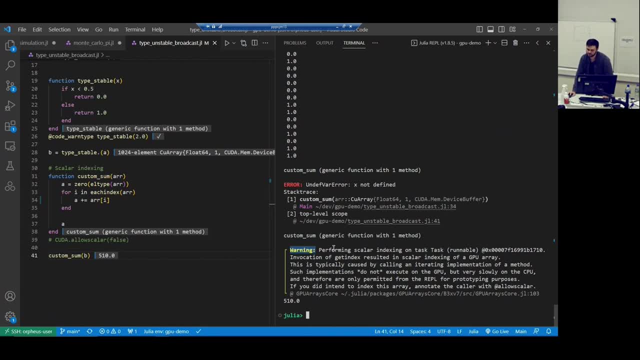 it does work here, but it gives me a big warning And it says that you're performing scalar indexing. So scalar indexing is when you have the array and you actually index and take one or maybe a few values out. And it basically says: 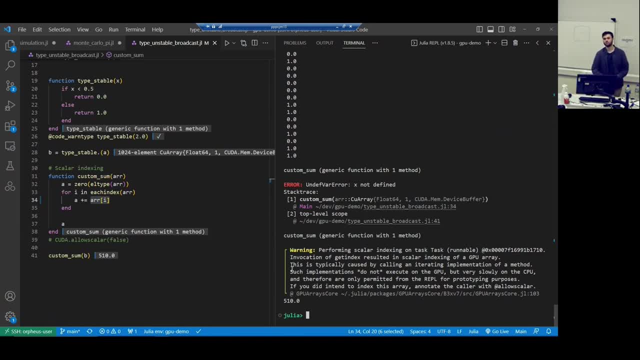 don't do this for performance reasons, And the main reason is you're not executing this code on the GPU. This code is running on the CPU, But what happens is when you try and index the GPU, it says: oh okay, I have to ask the GPU. 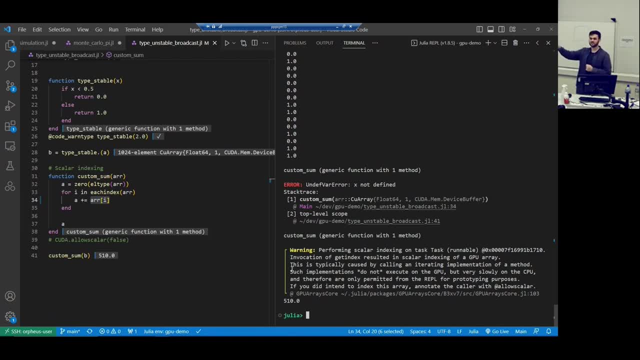 what was the value of this array at this index? And then the CPU goes and fetches that value from the GPU, goes all the way back to the CPU and then gets processed afterwards, which is a huge latency. And this happens every single time. 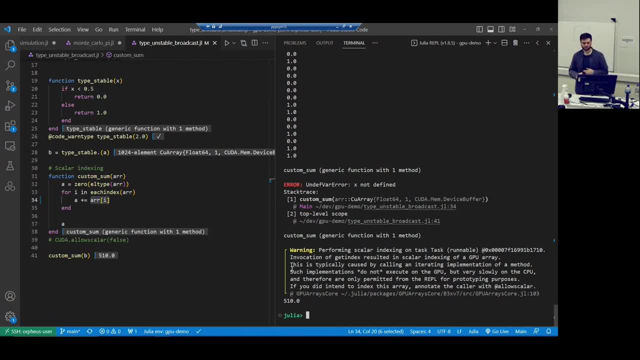 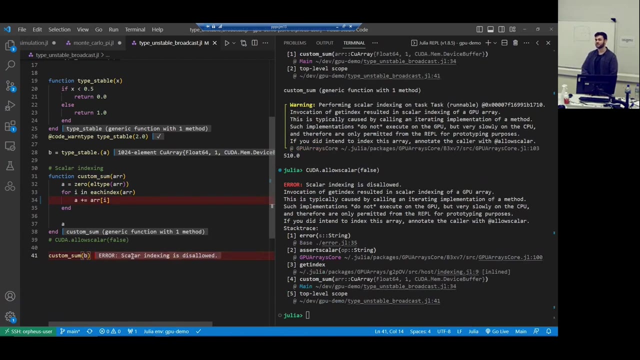 for each of the elements in your array. So usually what I would recommend is there's a function called cudaallowState and if you set that to false, if you try to run this function, it'll actually give you an error saying scalar indexing is disallowed. 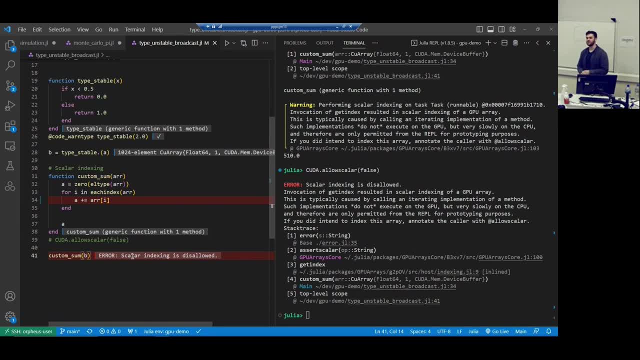 because almost 99% of the time you don't want this to happen in your code. You're moving to the GPU to try and accelerate your code, not make it even slower. Sometimes you might want it so you can use an annotation. 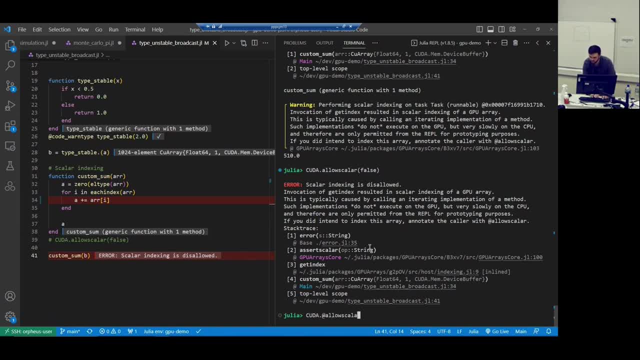 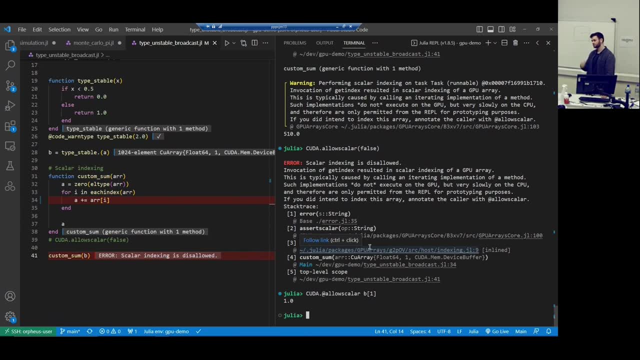 again from the cuda package called allowScalar, And so now you can index into that array. just fine, This is on GPU, indexing on the GPU. So this runs on the CPU, but when you get the value of the index it will ask the GPU: what is that value? 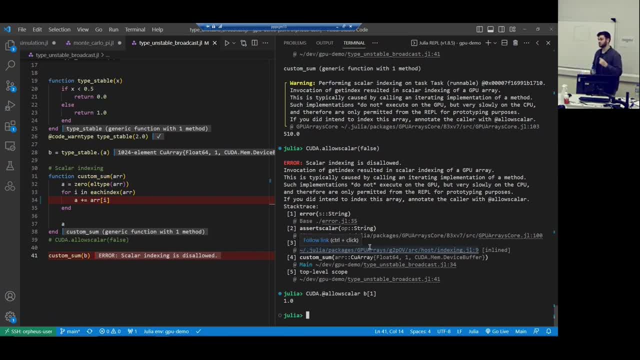 and then send it back to the CPU. Yeah, so that trip. the latency that it takes to get from the CPU all the way to the GPU and back is incredibly high. instead of just going into memory, Is there any way I can copy this? 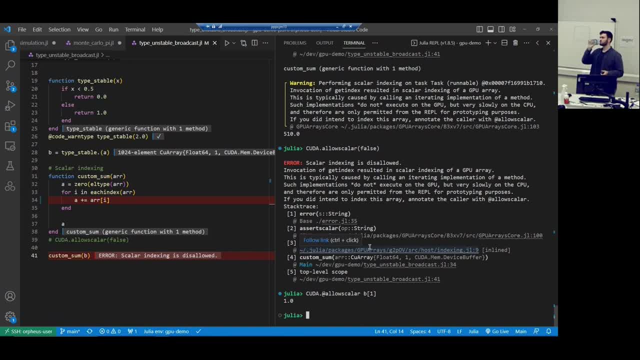 Yeah, you can copy this. You can copy this GPU array back to a CPU array: Mm-hmm, mm-hmm. So yeah, a lot of the time if you have a sort of small array back where it's faster to just do the operations on the GPU. 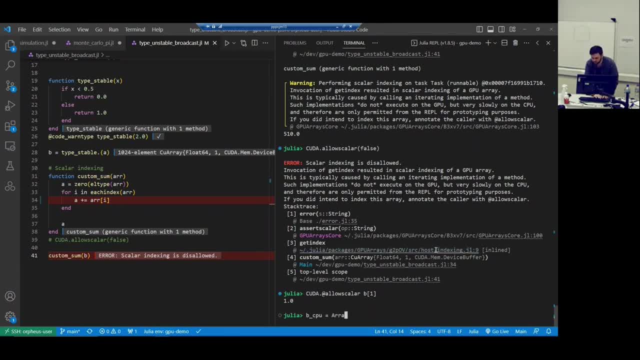 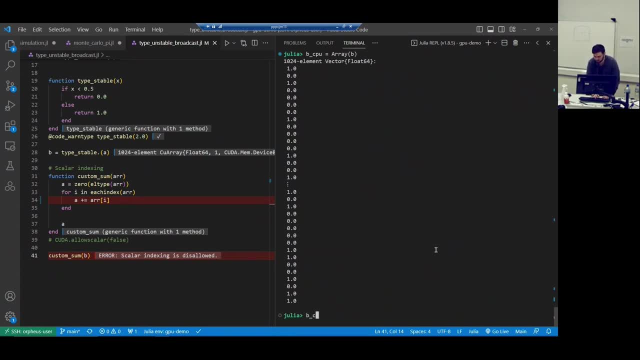 you can, for example, copy it and you just convert it to a normal array type, So you can convert it there, And then this bCPU you can use as normal. You can use your for loops and everything. So yeah, basically the conclusion is: 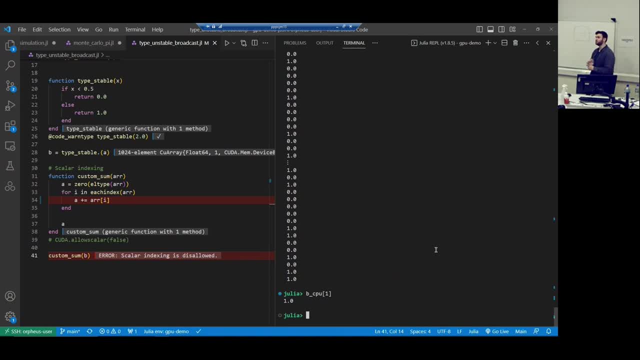 anytime you're doing the scalar indexing, so a for loop, your GPU code probably won't work, unfortunately. So if you're trying to write code that will work with GPUs and CPUs at the same time, if you can write it with broadcasting, do. 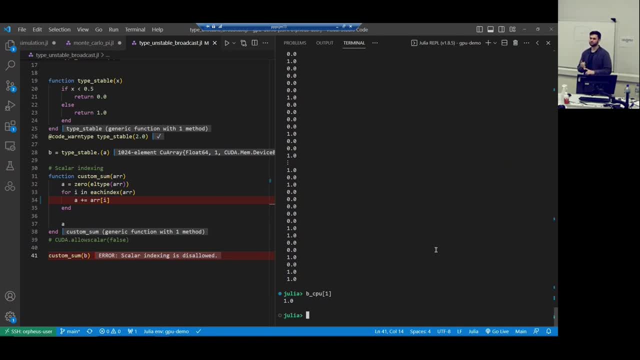 Write all of your stuff in, like the broadcast notation, use, map, reduce, map, produce as functions, and it should work for both, And all you have to do is just copy and paste And all you do is change your input types and you'll get implementations. 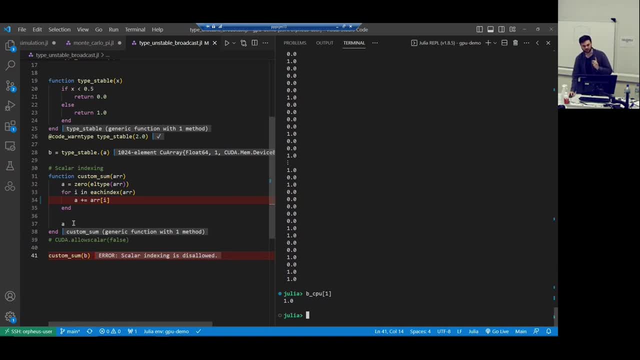 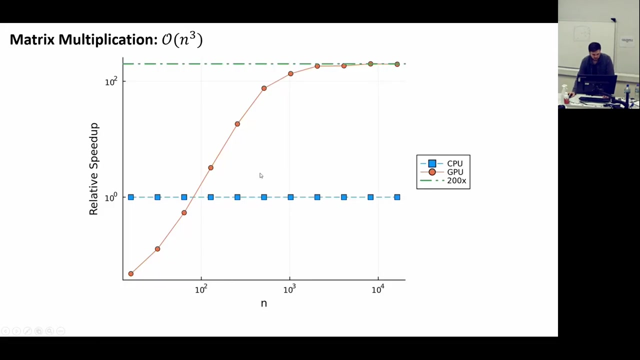 that are correct for CPU and GPU. In the cases where you can't and you actually need these indexing in some way, you can write your own custom kernel And we'll talk about more. we'll talk about that more next week. So if I go back to here, 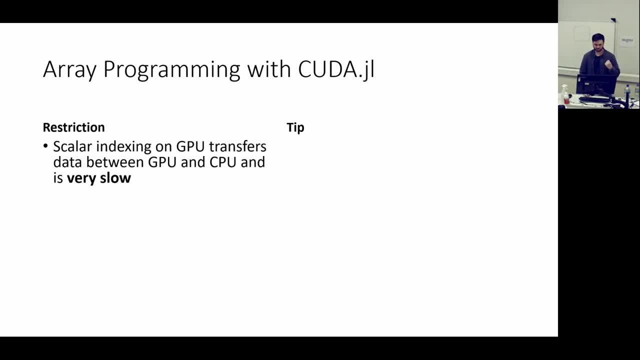 I'll just sort of summarize what we've seen in the examples. So big one, Big one is scalar. indexing is very slow, And so you don't want to be transferring data between the CPU and the GPU for each element of your array. If you need to do it in some way, 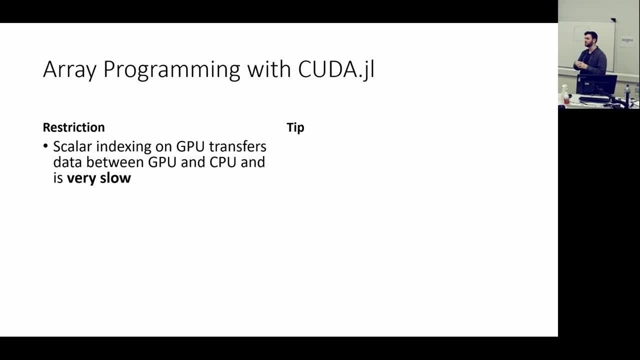 it's better to do what you suggested and copy the array back to the CPU and then do all the processing there. Copying that doesn't destroy the GPU array, right? No, copying doesn't destroy the array. It stays on the device memory there. 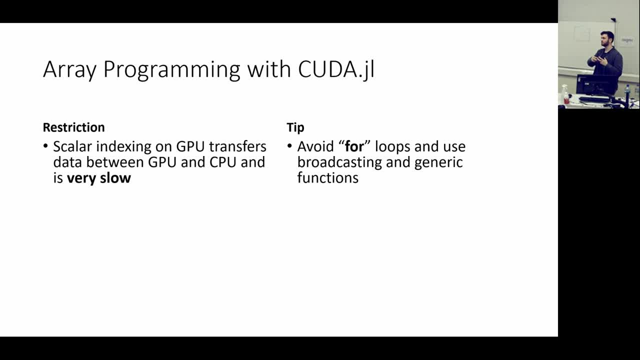 But if you change it on the CPU then the device memory will be unchanged. So the only way you can see those changes is if you copy it back. So yeah, the way to avoid the scalar indexing if you're trying to stick with the very sort of 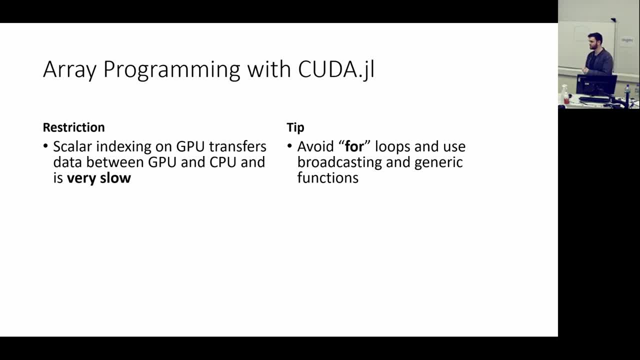 high level array-based programming is: avoid using the for loops in your code. If possible, switch to the broadcasting notation and use these sort of generic functions, As I listed before. Again, if you're doing any computation on the GPU, the memory that you're operating on, 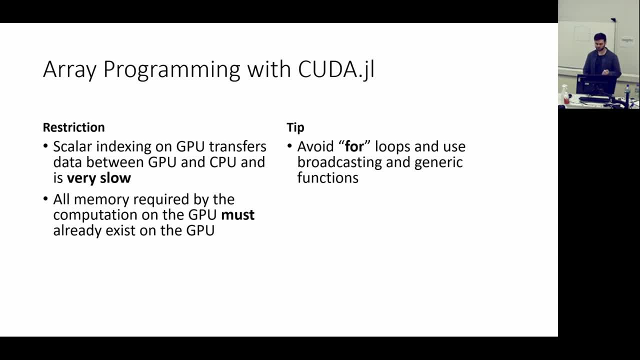 needs to exist on the GPU first. So essentially this means creating your GPU arrays And if you want sort of high performance, instead of allocating an array every time you want to do an operation, you can use these in-place operations. So, like Molbang, the broadcasting dot equals. 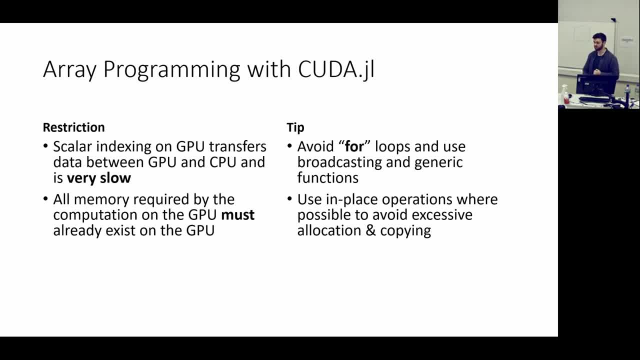 to avoid having to allocate a lot and copy data around a lot as well. Usually, what happens is in a pipeline- is you create your data possibly on the CPU, copy it to the GPU and then keep as many of your operations there as possible. 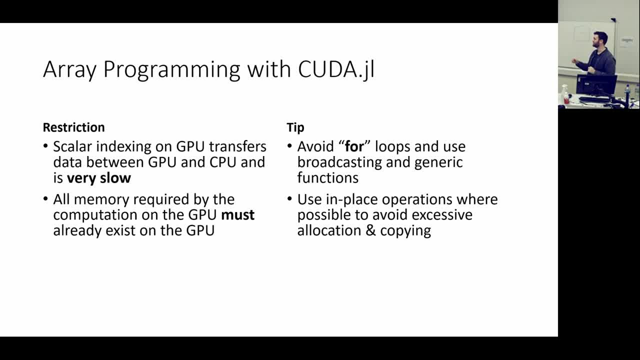 instead of having to copy back and forth. That's sort of your last resort strategy. is you want to avoid having to copy back and forth between them Again? any use case, Any functions that you use, must be type stable as well to be able to compile to the GPU. 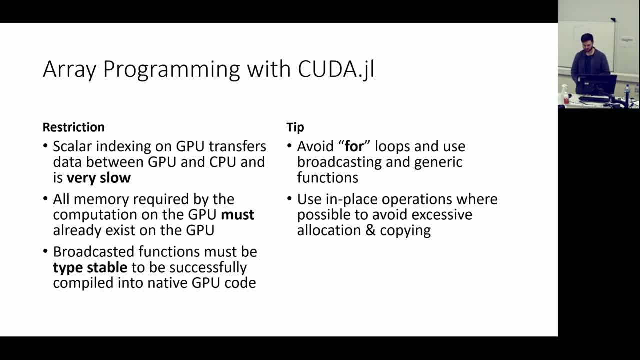 We'll talk about this a bit more on Thursday as well. For now, just use this code: one type macro. probably get into the habit of using it anyway for your normal code, because it's also good for CPU performance to make sure everything's type safe. 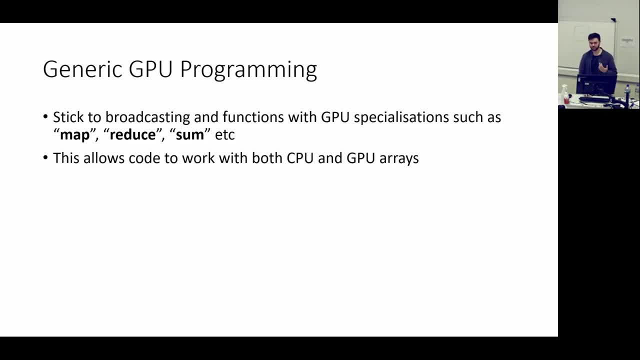 Okay. so if we want to go to sort of generic, so being able to do as much as possible on the GPU, Again we can use the sort of generic functions that's fine. But if we do need this sort of more complex behavior, 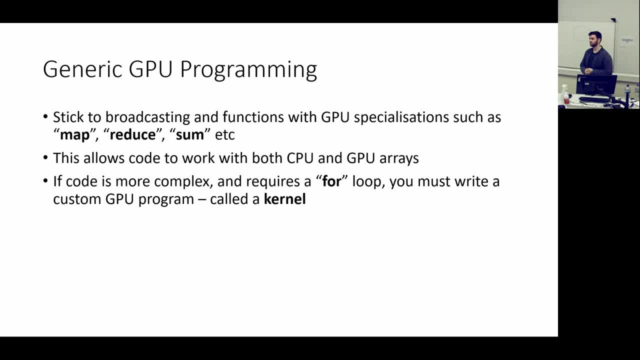 that you can't easily achieve with broadcasting. you can write your own kernel. We'll go over exactly what that means next time, but this is essentially mimicking how you would write code for the GPU in a language like C that doesn't have this sort of very nice 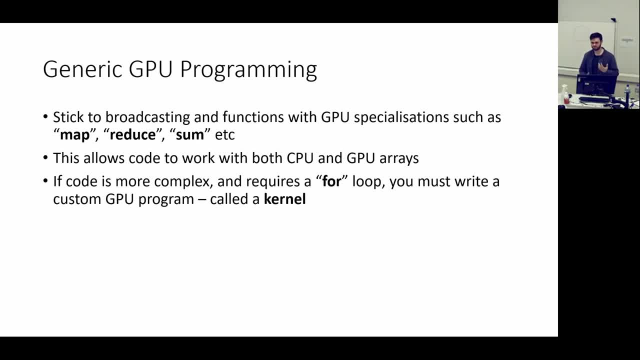 high-level array-based API that you can use to make your code very generic. Yeah, I didn't go into too much detail about this, but we wrote our own native Julia code and that got compiled into something that ran on the GPU, So it's already generating these kernels for you. 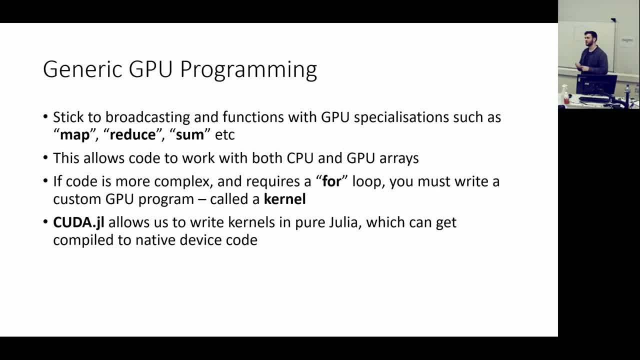 from the GPU code, but in a very specific way that fits with, like map broadcast, reduce all of these, all of these things, But that's the sort of high-level wrapper around actual real kernels. So we'll talk about that next time. 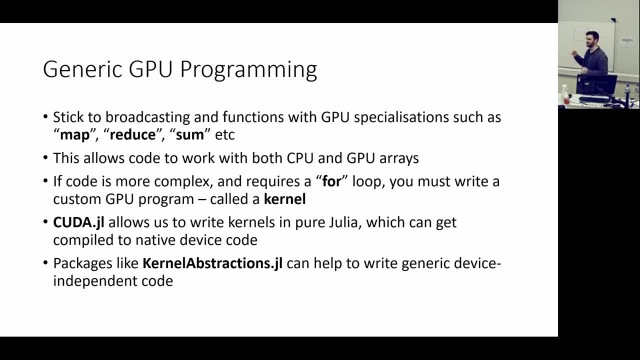 Yeah, there are some packages that will go over making this kernel writing process a bit easier, and it also lets you write kernels that work on CPUs, GPUs of different brands as well, So like NVIDIA, AMD, Intel, et cetera.